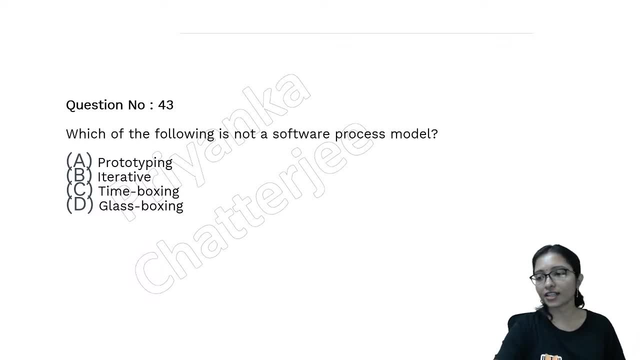 be the answer. Yes, you learnt this, all the topic. Now tell me what will be the answer of this question. Okay, everyone is here, I can see you. Sekandar, Deepa Lakshmi Varti, Asha Ashok, SHR. Vanja Vanja, Muthayan, Darpan, Aspya, Venu Lekha, Sri Ramaya, Divya. 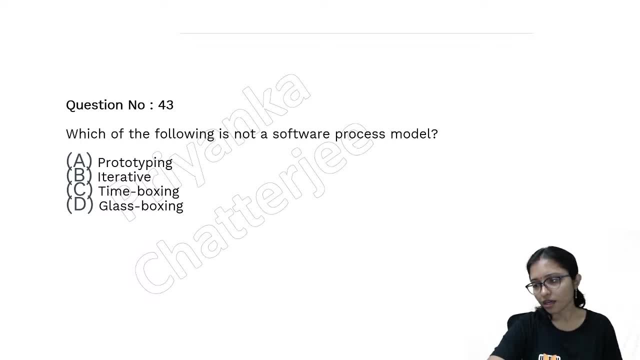 Sneha, Rajnikanth, Vishwapriya, Rubiya, Kaila Maritha, Kaila Kaila, Kaila, Kaila Kaila Kaila, Daniels, Dinke, then Ishwari and Vabani, Josh, Vetri, Sarnalipsha, Praveena and Gopinath. 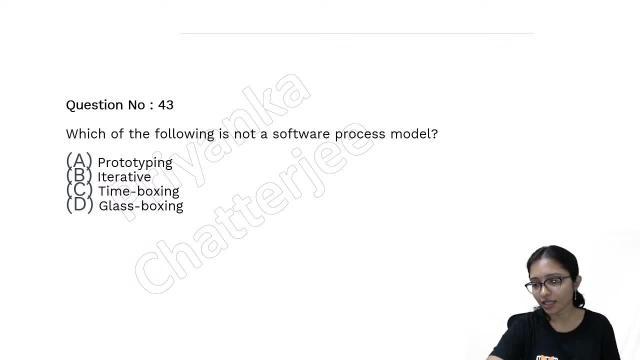 Priya, Ammu, Aj, Remove ajb money. come. all are here. yes, all of you are telling the answer is d, d, d, d, d, c and d. no, c is not the answer. answer is d time boxing. time boxing is also one type of software model. it is asking. 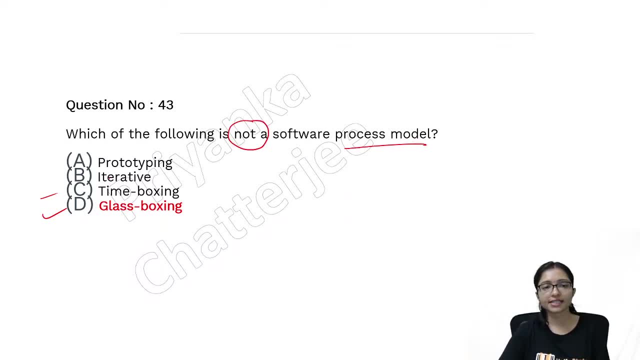 which one is not the software process model, that is, glass boxing is not the software model. time boxing is also the software model where we are dividing as per the time. this time, we will do this work. this time, we will do this work, okay, okay, raja lakshmi, yes, raj lakshmi, hi, now tell me what. 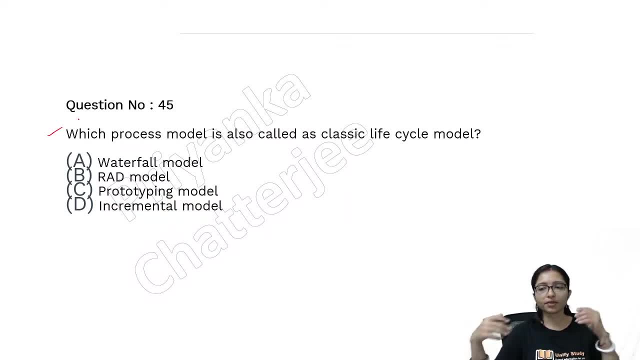 will be the answer of this one: do quickly, quickly do the previous revision. after that we will come to the agile method. always. i will ask you some question of previous topic, then we will go for the next one. do this one, do this one quickly, which process model is also called as classic life cycle model? 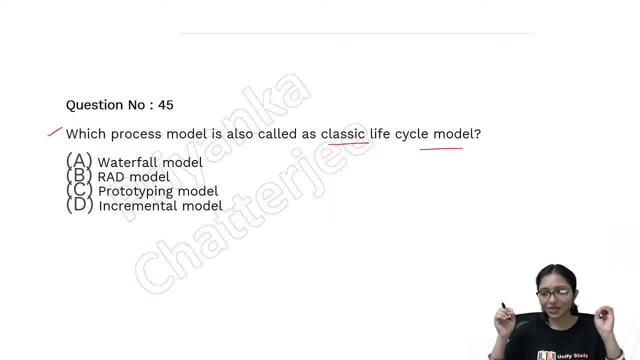 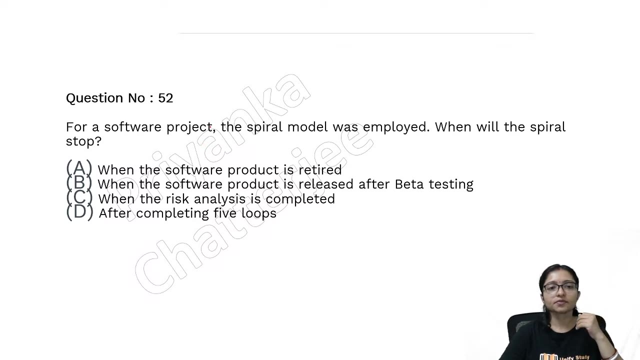 yes, yes, quickly, quickly answer quickly. okay, all of you are giving correct answer. yes, classic model is waterfall model, next one, next one, do this one, oh, do this one for software process anyット, okay, okay, this one is also very important. if we will do this, sit, let me write down. 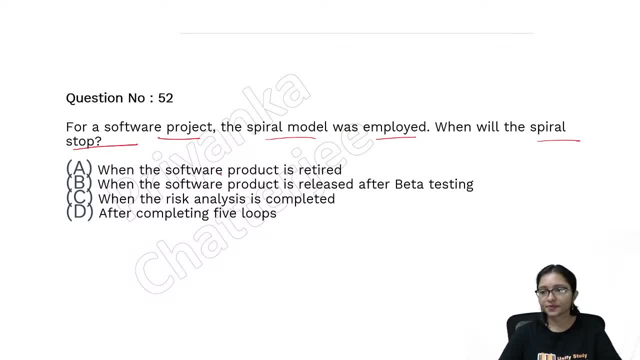 a lesson if you will give your answer yes. yes, these are the questions n, because i have collected from different. there was 100 mcq, so from there i have collected according to this topic. so forgot about question number. just focus on the question. okay, answers are coming. 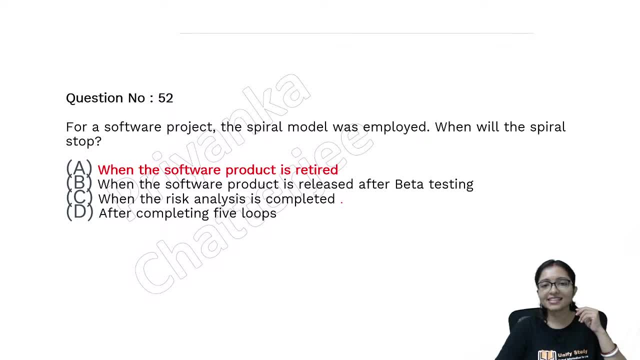 so you are giving answer that when risk analysis is completed. that is wrong. that is wrong. when software product retired means ultimately software product are not now it's not able to work. that is only otherwise whole full the life cycle. the risk analysis will be there and full the life cycle. 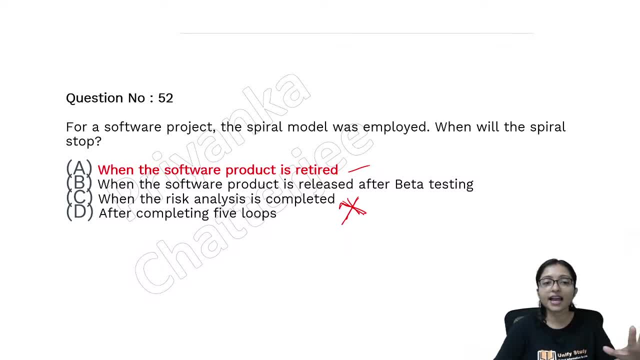 spiral model will work when it will retire. software product is not working more. it's retired, it's taking retirement, then only it will stop, otherwise it will not stop. so answer will be a: when the software product stop, then only it will retire, then only spiral model will stop. okay. 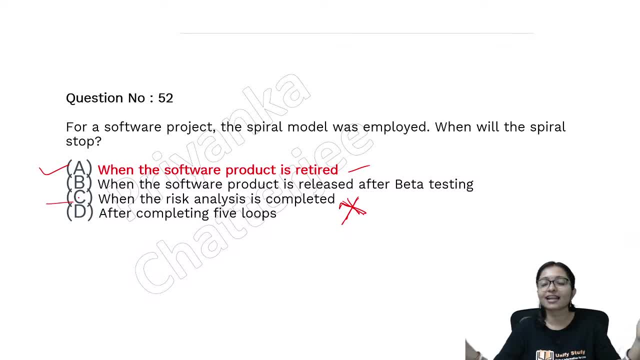 okay, most of you are giving answer. see, when the risk analysis risk. always, always there will be the risk. whenever you are working, there will be risk. when you stop working, then there is no risk, no risk, no gain. right, so no risk, no gain. that's why, whenever, whenever you are working, then this: 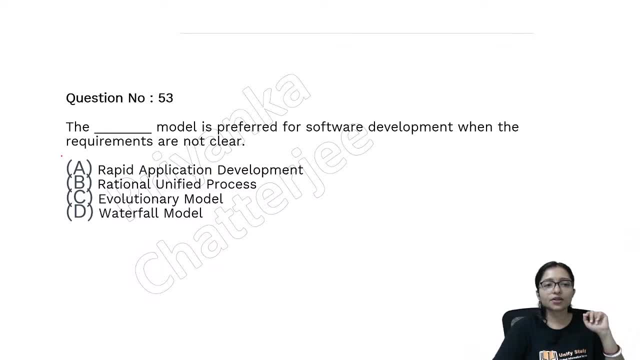 will be there now. tell me what will be the answer: the model, the dash model, preferred for software development when the requirements are not clear? when the requirement are not clear, what software model we should use? yes, question you have to do in my class always remember i will. 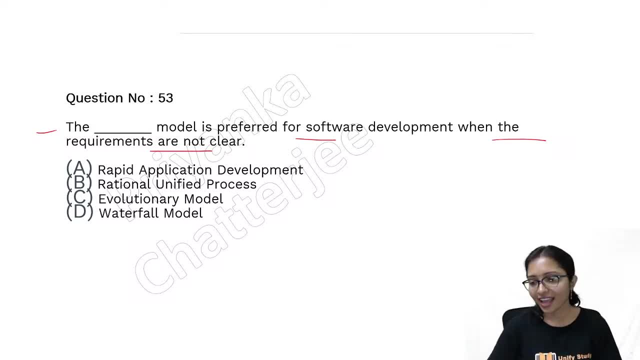 teach you topic and i will ask you question. i will ask you question, thank you. thank you, rohit. thank you, try to increase unified study family more. thank you, yes, yes, that is here. here it's evolutionary model, because yesterday i told that evolutionary model is one type of prototype model. right yesterday i told that evolutionary model is one type of 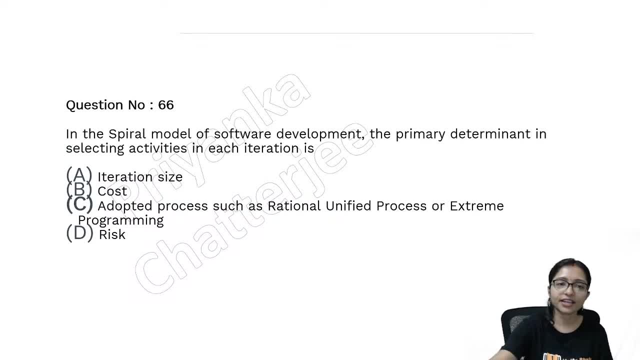 prototype model so we can go for it. very good, all of you, you are doing study. well, that's good, that's good. here. now do this in spiral model, that this is very easy question, super easy question. this is very easy, super easy question. do this one so. 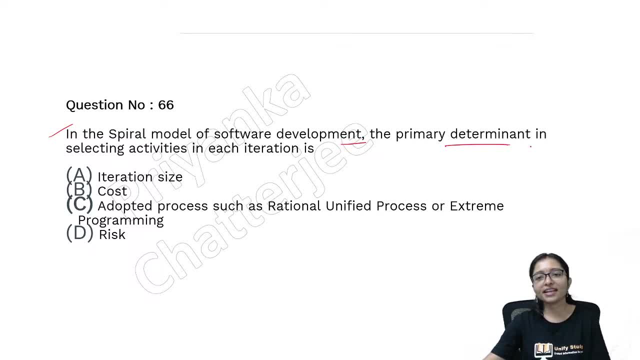 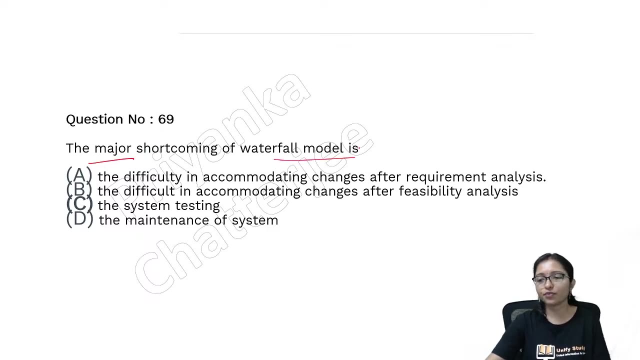 yes, easy, one right, spiral model, primary determinant of the selecting activities in each iteration. that is risk only, it is following the risk. very good, very good. now do this one: the major shortcoming of waterfall model. what is the major shortcoming of waterfall model? good, good, good, very good, everyone, everyone. 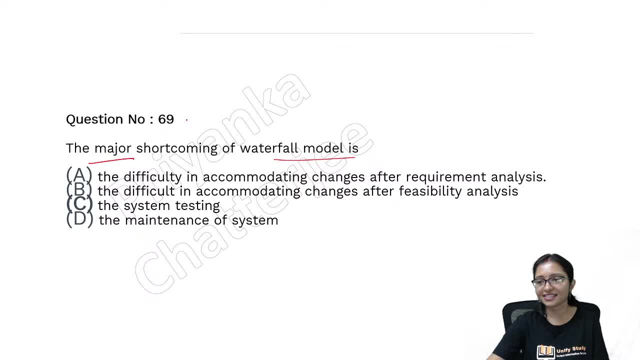 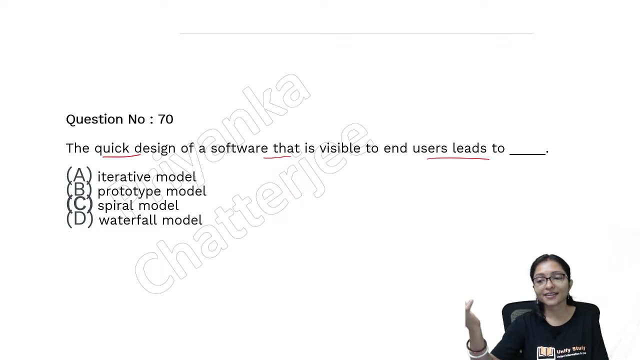 is doing correct. now tell me what will be the answer of this. yes, yes, answers are coming. difficulty in accommodating the changes after the requirement analysis. this is the major shortcoming. yes, very good, very good, all of you. now the next one. the quick design of software that is visible to end user leads to what? but which model? which model? 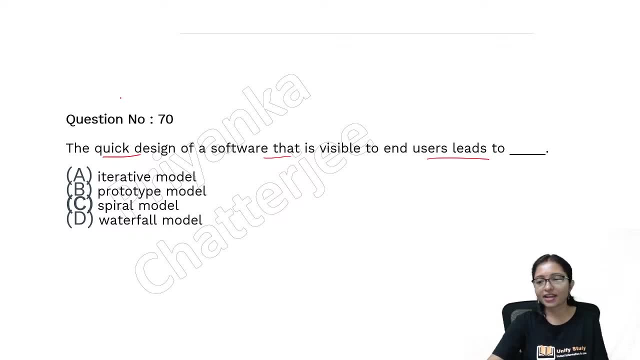 we will go for it. do this one. what will be the answer for this? don't focus on question number. okay, i am giving the specific question for the specific area, so i copy some copy from my another slide. that's why question number is showing, so don't focus on question number. give me the answer you can answer with. 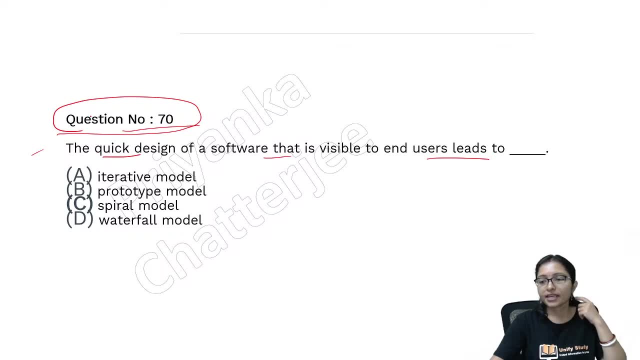 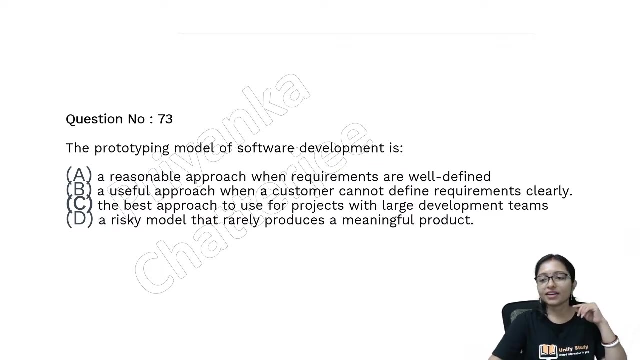 the question number also. that is okay. yes, answers are coming. yes, very good, that is prototype model. definitely when it is not visible to the end user, that is visible to end user, that is prototype model. very good, everyone very good. the prototype model of the software development is: 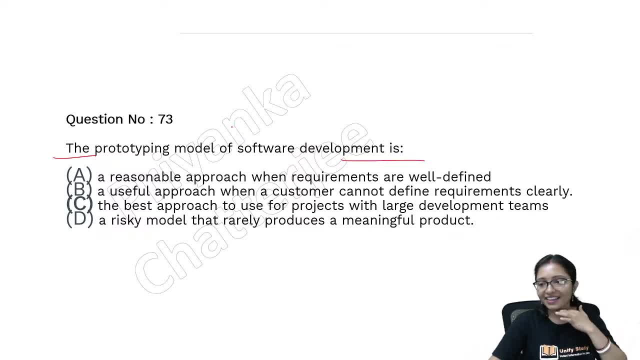 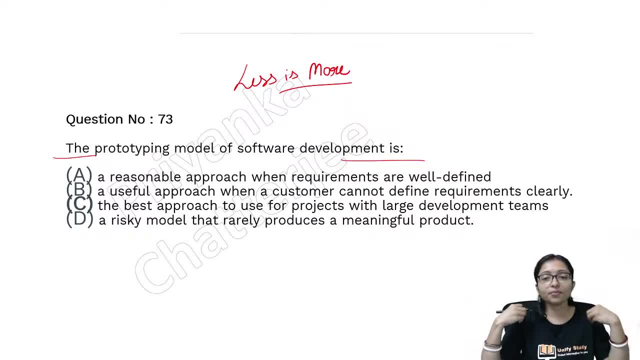 do more practice, less consuming, more practice. right, i will do the lecture, lecture, lecture. you will not practice, that will be not good. you have to practice more. yes, answers are coming very good. b is the correct answer, b is the very, very good. the user, the useful approach when customer not defined. 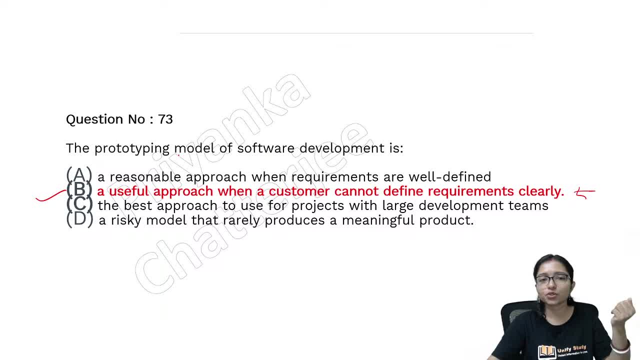 requirement. clearly, then, we are going for prototype model. very good, all of you. so, yes, pakka, now i can tell you that this way, this course is very good. that is to be taught theנס, not goodyeah. that is very good, understand. yes, my teaching was correct and appropriate and you learn also appropriately. 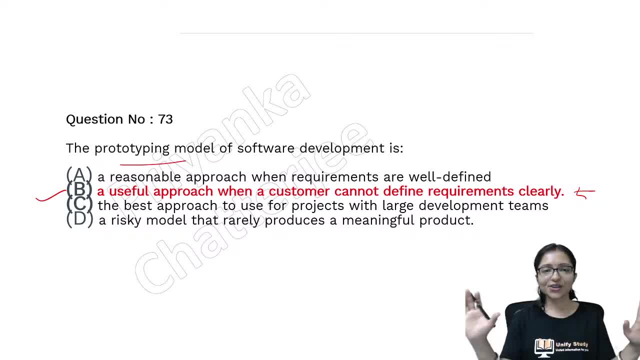 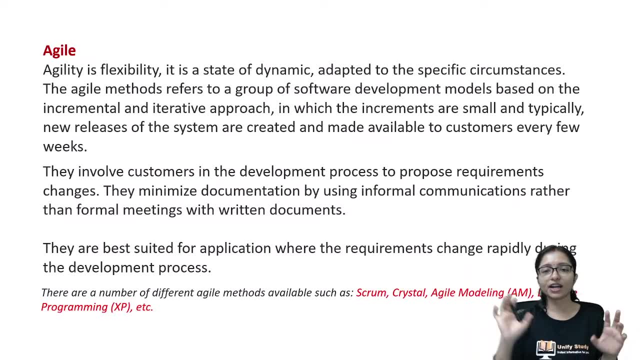 now. because of that you are able to answer right. so, sdlc, whatever we learn till now, that is very clear to everyone. so congratulation, you learnt one topic. congratulation to you. you already learnt this topic. now we will learn the azil method. so yesterday we did all that topic. now 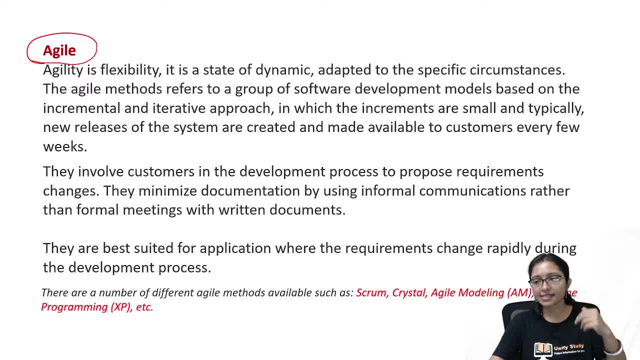 we are going to learn the azil ideas again. also because of that, we will deal with them during the while methodology, because before starting agile methodology, if you don't know what is waterfall model, what is prototype model, what is iterative model, what is incremental model, then you cannot 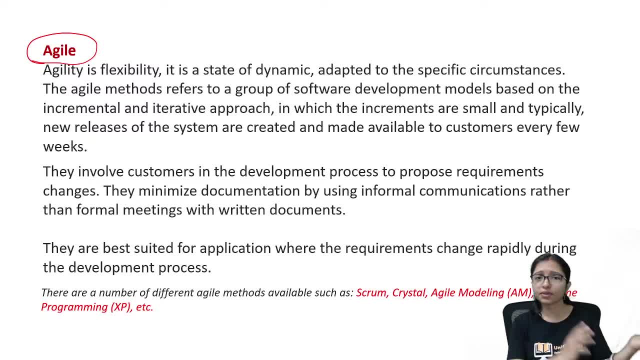 do agile. so if you did not watch the previous one, then definitely you have to watch the previous one. then only agile model will be clear. yes, so agile model is nowadays agile model, is very, very super active model. everywhere it's using agile model. so agile philosophy, but it is the agile is. 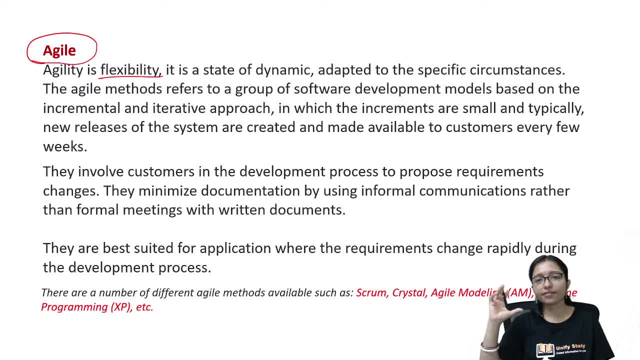 the flexibility. flexibility is important, right any time. any change we can do. that is giving you that flexibility and state of dynamic adopted for the specific circumstances in agile method. what are the main focus of agile? i am telling you as we are. whenever we are going to build a software, some of the requirement will be clear to us definitely. 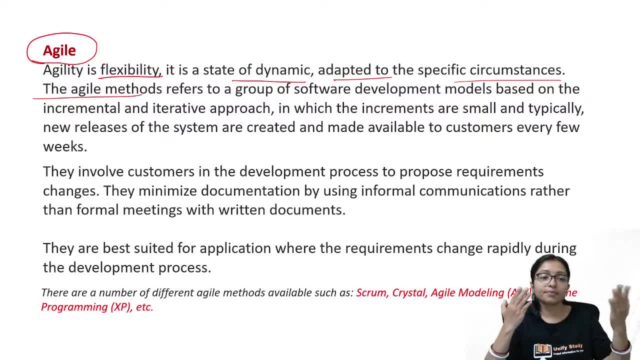 day by day, we can understand that, yes, this is may be required. that is may be required at the beginning. if you are asking to the client that, tell me your all requirement, it will be very difficult and even also if you are waiting for that when completely requirement will be clear. 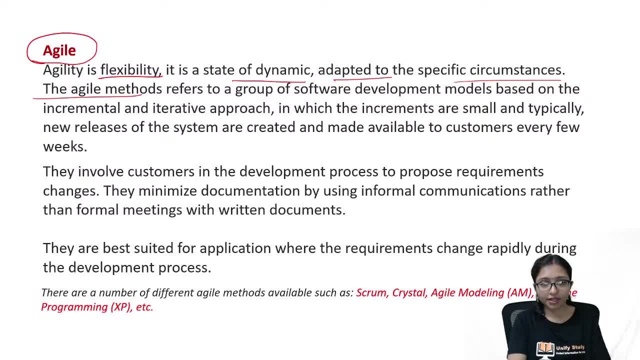 then only we will start. that will be also difficult. and too much documentation, too much documentation. ultimately it's a it's a wastage of time. too much documentation, previous model, what is waterfall model and other model- too much documentation is there. they are spending lots of time for documentation of requirement. so, as i is doing like that, okay, it will do and it will do the. 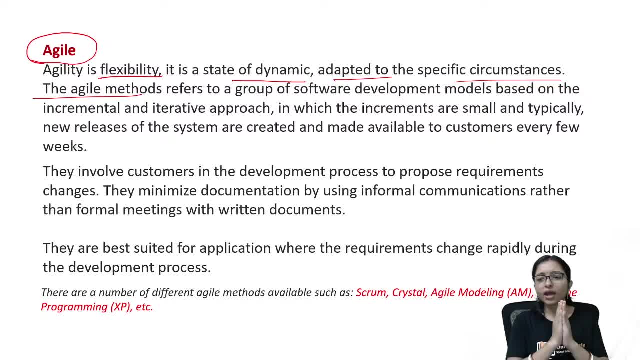 meeting with you customer, some of the requirement will be clear. after that they will start development. they will not wait that okay, i will confirm everything then. only i can start. no, so that's why it is the combination of incremental and iterative approach. yesterday we did incremental and iterative. 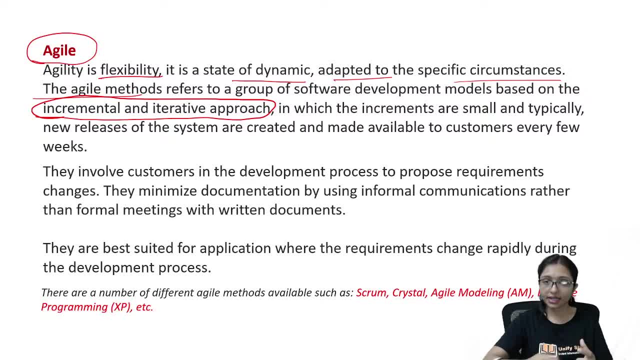 it is a combination of incremental and iterative approach. that is the process. one is set that which increments are small and typically new release of the system. so here there are hundred feature out of hundred feature may be 10 feature. i will do out of that 10. 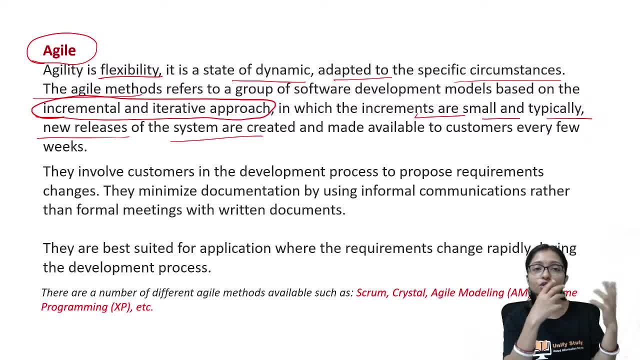 feature also. i am not doing completely out of that 10 feature also may be 20, 30, we will do. that is the concept of combination of incluemental and iterative. there are total of 10. so so now the There are total 100 feature. 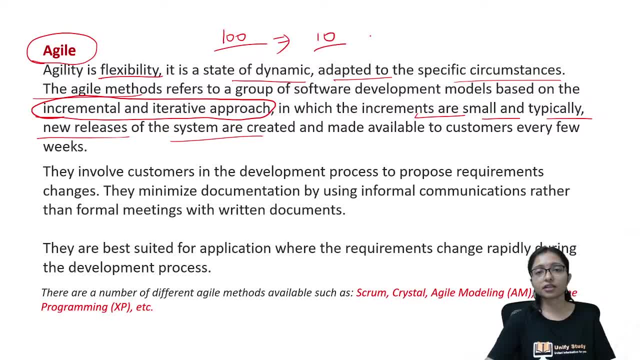 First iteration we select, we will do 10 feature Out of that 10 feature. also the feature 1, we will do 50%. Feature 2: we will do 70%. Feature 3: we will do maybe 60%, Like that way. 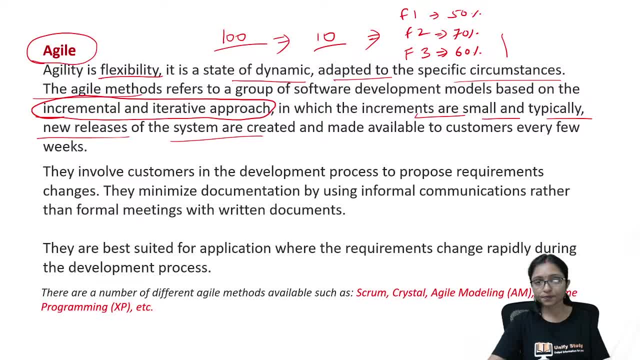 Like that way. That's why it is the combination of both: Okay, So created and made available to the customer very few weeks, Very quickly. we can create it and we can make it available. That is that is I did. Actually, I did that one. 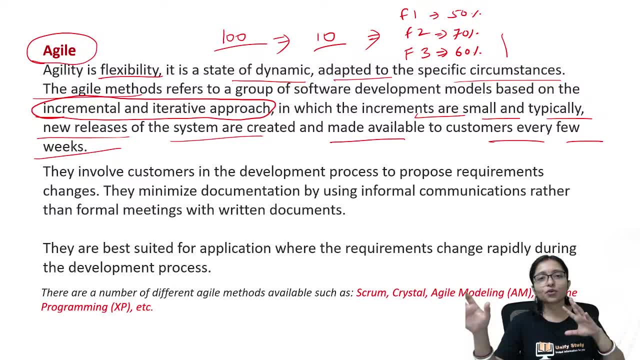 You do that? yes, ma'am, that is not working in app. That is not working. It is not there. Ma'am study material, Ma'am mock test, Ma'am live class. So I did not wait for that, Because I know that if I am waiting for that, then app I cannot launch quickly. 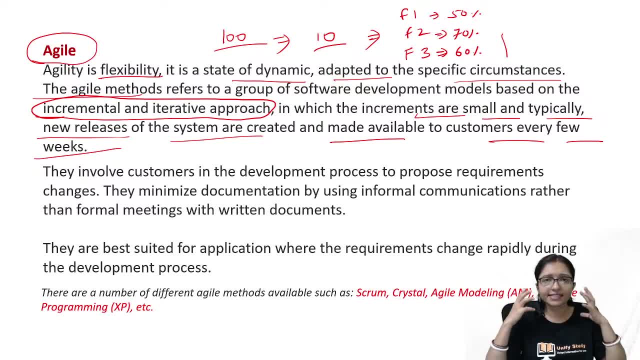 My target was that. okay, It was a very sudden decision. Really, it was a hard decision For me. that is very quickly. It was totally unplanned, As I just as I will have a unplanned thing, Whatever happened with me. that is also totally unplanned. 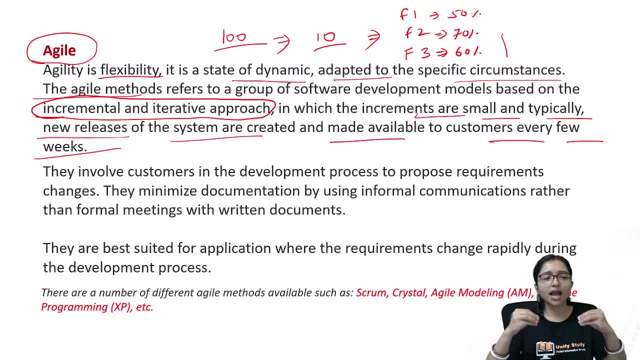 Exactly on 14th August. also 15th August also, I was taking class. very happily, I was so happy I took the class Even. also, it was not known to me It is going to be happen at night, But when I saw that at night, 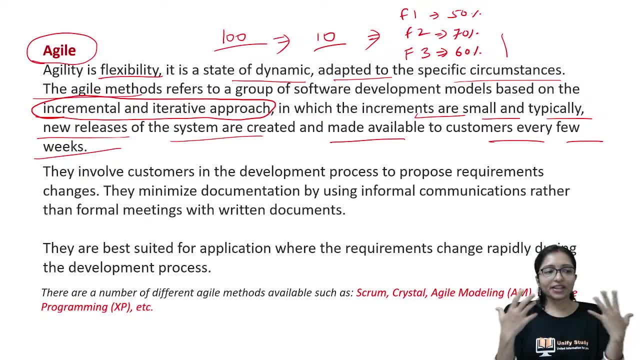 Oh, my God, What is going on? So that Whenever I saw that there are some policy but I cannot agree anyhow, that was totally unplanned to me, suddenly what I can do. so suddenly, very quickly, I have to do something very quickly, I have to do the decision. so I cannot wait. I cannot wait. that is not possible, right? so that's why what we thought, okay, go for as I methodology, do some short thing, some small feature, try to develop the small feature and and. 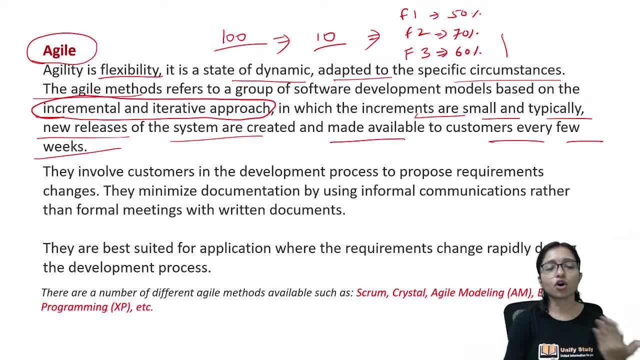 Publish it and after that we will work on it. after that we will, later we will work on it. that is, that is the advantage of as I methodology. that is the very much means we apply. now we are applying as I methodology for unified study app. really now we are applying even. also, website is not till now integrated that much, and the Android, iOS version and so many things are there to do. 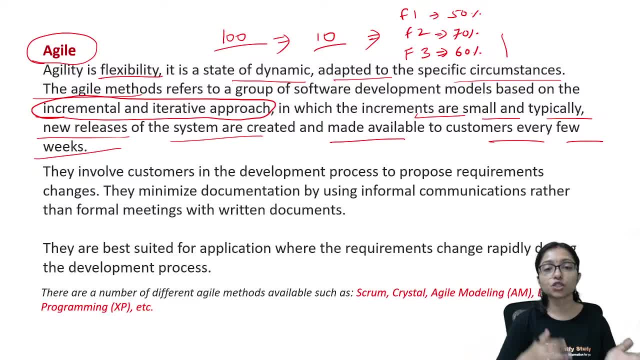 But still we started. yes, we cannot pause. we should start for a long time. we cannot wait. that is as I methodology, and here customer involvement is very, very important. the customer involvement, member customer involvement, by every day there will be team meeting. I am also doing with the doing- meeting with the team every day. it's for a, not a for a for formal way, it's totally informal way. 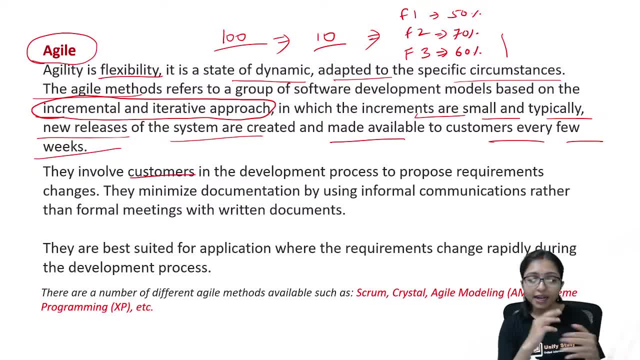 It's not like that. I will send mail. they will reply and all know, just like a WhatsApp. in the WhatsApp I am sending message: this is not working, that is not working. they will reply if required. for 10 minute we are doing meeting and we are discussing. okay, this is the way we can go ahead and they are doing work. it's totally very friendly environment, as I is giving you a friendly environment where developer can work. 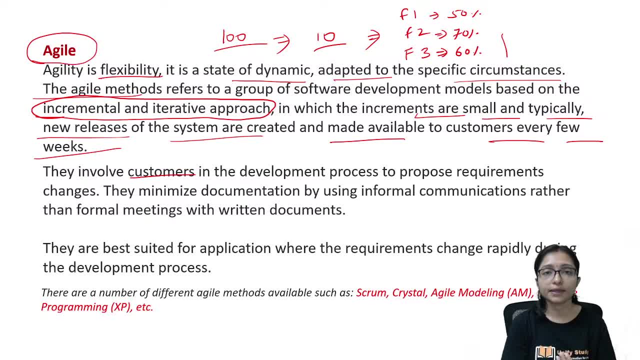 Friendly and customer will be also friendly with them so that both will be very much comfortable in that area. that comfort zone will be there. if it is total, process oriented as I is not process oriented as I is people, it's focusing on people, not the process, because if you are thinking about too much process, you cannot proceed. okay, if you are thinking about 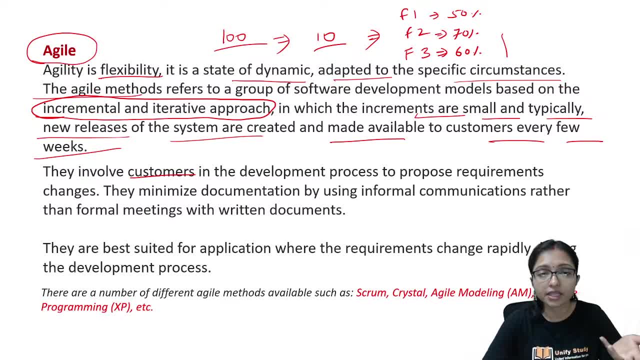 How I should. I should talk with the people so that they will feel okay, they will feel motivated. I am also trying to motivate my developer. yes, you are doing good and do this way. I am guiding you do this way because I cannot right now quote, but I am giving you planning. do this way so that they will be also motivated and they can go ahead. if you are giving too much restriction, then they cannot work. that is the advantage. 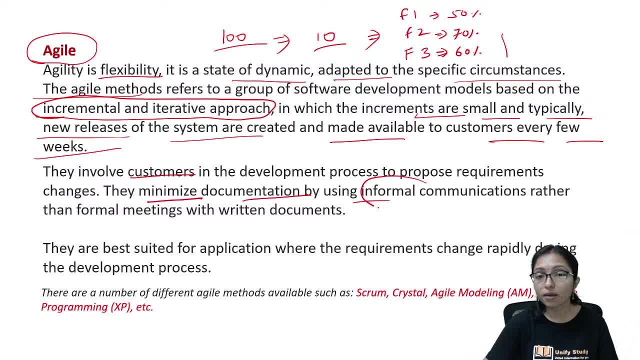 Minimization of document by using informal communication. it's not at all formal communication rather than formal meeting and writing document. there is no written document whatever. whenever I have started, till now, there is no written document. what is there? everything is going on in whatsapp whatsapp. there is a whatsapp group, just like that. in whatsapp whatsapp, everything is going on. 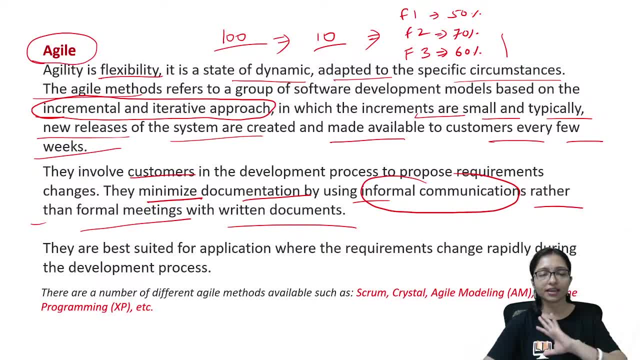 With us and I really happy with that. okay, my developer are working good, so here they are based, suited for the application where requirement changes rapidly during the development process. every day it can be changed. every day, anytime it can be changed, and that's why here the scrum, crystal, agile model, extreme programming. these are the some framework methodologies. 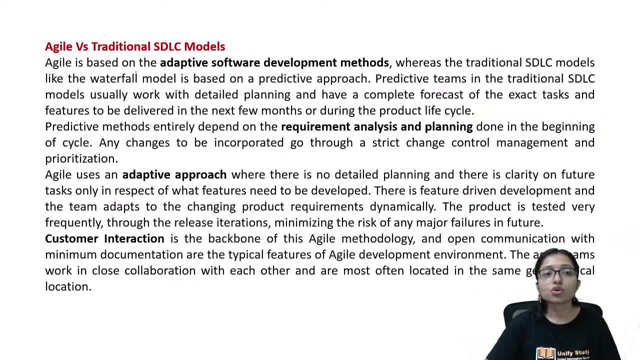 Is using here. okay, so what are the main difference between as I what? versus traditional SDLC? As I, based on the adaptive software development model, it is the adaptive. Adaptive means it is adapting anything it can, whereas traditional SDLC waterfall, based on predictive approach. adaptive means 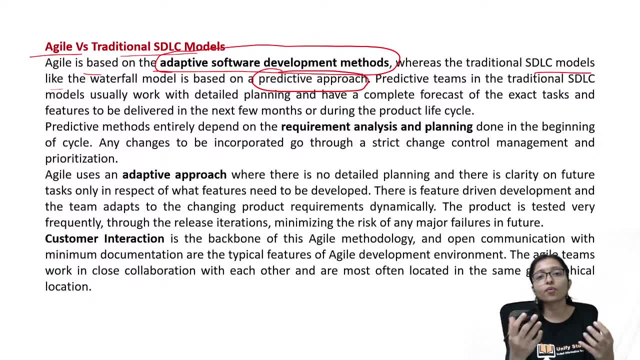 According To current scenario, what is required? we will do that. Predictive means it is trying to predict the future. in future it can be happened. then we can go to the door for this and we are doing like that. okay, whatever will be happened on runtime, we will handle it. 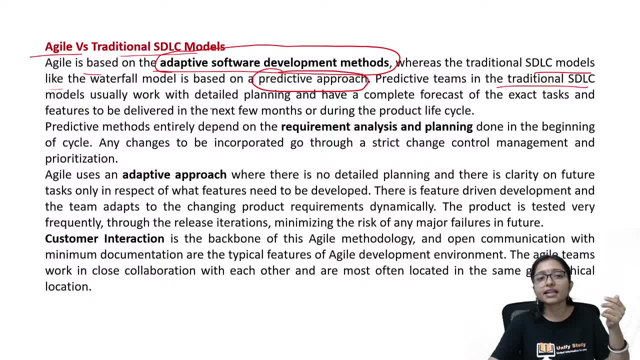 That is called adaptive Predictive team is traditional SDLC model usually work with detail planning. here the detail planning is required. Complete forecast is required. in today, today's scenario. I cannot say what will be tomorrow. I cannot say after one year what will be with the app. we don't know, so we cannot forecast it. 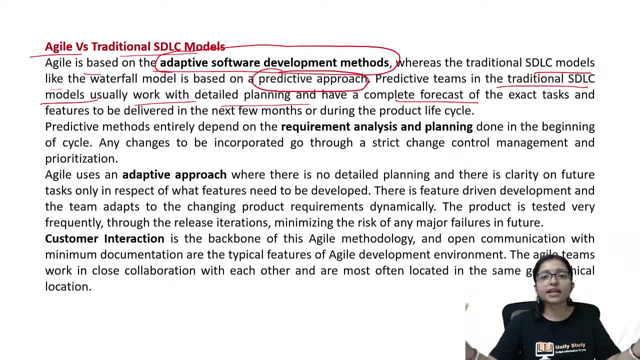 But we are thinking: okay, today it's expected 200, 500 student can be there. okay, we can support it after that. After that, what we can do if there are Thousand, Two Thousand Students are coming, according to that, we will try to support. 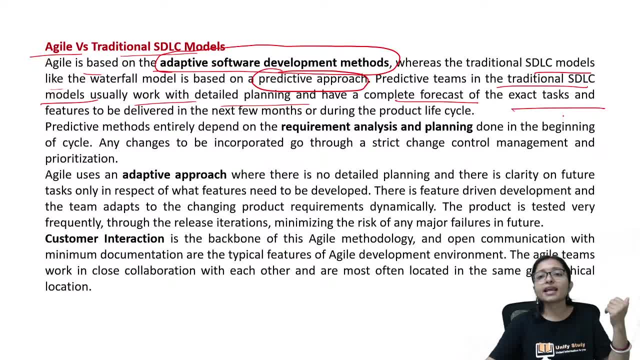 Right, so we cannot forecast anything. so here: exact, exact text: feature delivery: new few month during the life cycle. Okay, this is the main thing: requirement analysis and planning. I told adaptive approach- remember that this is adaptive approach- and the customer interaction also. customer interaction is the backbone. Of Agile methodology. everyday customer has to be involved with the team and as I am a computer science and as I am a IT developer, as I have that IT development knowledge, so, like me, if the customer is there, then so it is more, then so it is more. everyday I am interpreting: yes, this is like that. no, in database, that type of changes should be required. no, the locking should be required. 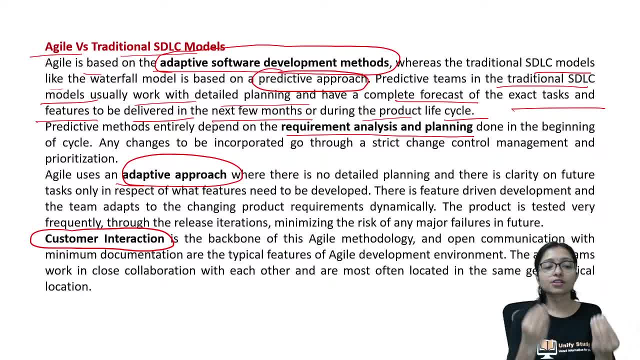 This is like that. no, in database, that type of changes should be required. no, the locking should be required. no, the locking should be required. But you should validate that every day. I am guiding them because customer interaction is a big part in agile. okay, here you can see that peace. 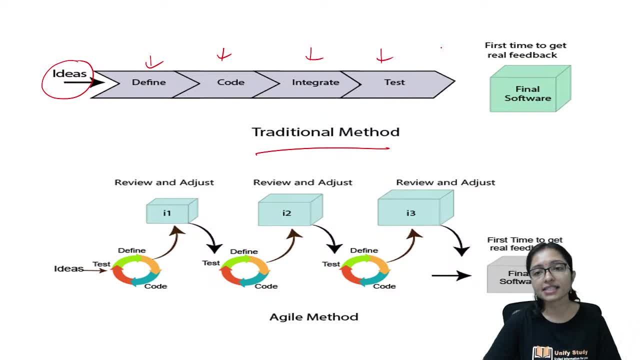 Acti. Here you can see that traditional method. normally there will be the ideas after that: define code, integrate taste, give it final. we are doing. but first idea: we will take small things we will do. after that they deliver it to me, they will put something in it there, send all. 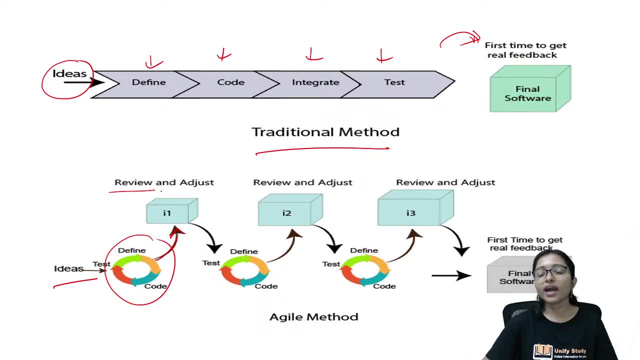 Egypt. they deliver it to me. after that i review and adjust. i told them: no, these are the, some changes are required. again, they send again. they did it, define it, test it again. they send me: okay, this is the thing. again i review and adjust again. it will be given again. review and adjust again it. 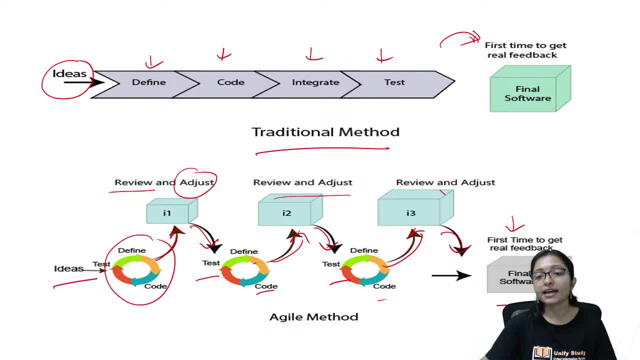 will be given like this way, ultimately, final software will be ready. this is the advantage of agile methodology: every time customer is involved. otherwise, what will be happen? maybe you are developing it for 90 days. okay, you are not asking anyone customer, is it okay or not? after 90 days development, you are delivering it to customer. now, customer is telling you: no, i am. 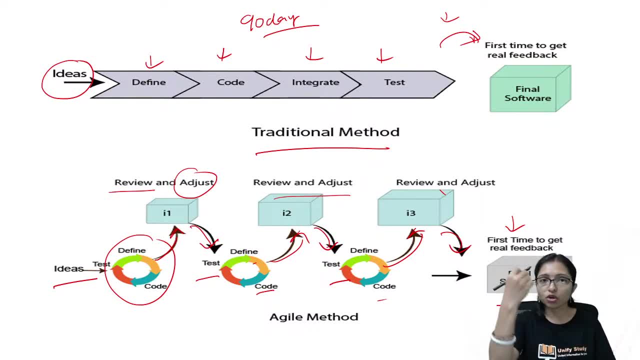 not happy with that. i am not going to take it. so your 90 days is waste. your 90 days is completely waste. rather than that, these 90 days, if we are dividing into three to four weeks, means one month. every one month, we will interact with the customer. i will send it. whatever we did, we will send it to customer. 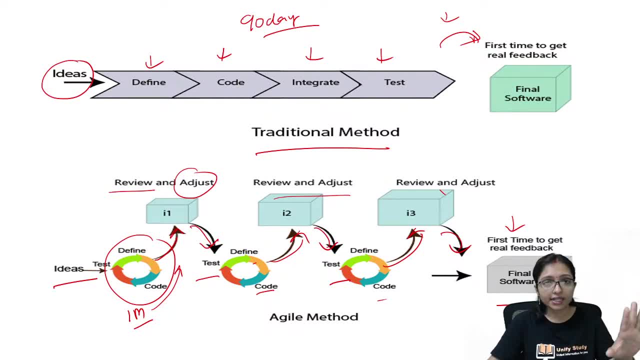 customer will check it. okay, what is thing, what is the required to adjust and what are the changes are there? customer will send us: yes, these are the changes. then again, next one will be done. that's why it is more good way. there is risk also less. risk also less, because every time customer is involved here. 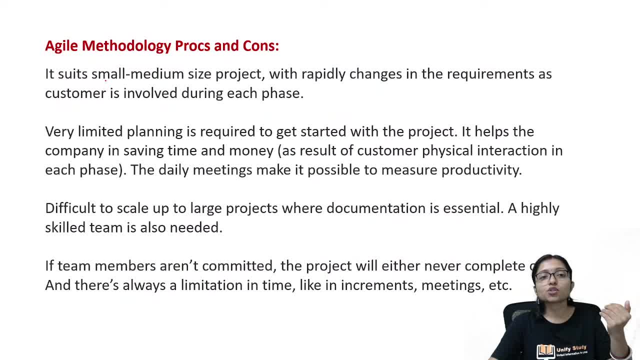 right, got it. so here suit for small, medium size project. it's not for good for the very big project. rapidly changes- that is very important part where rapidly changes of the requirement as customer is involved during each phase, then we will go through. very limited planning is required and started with the project limited to scale of the large project. 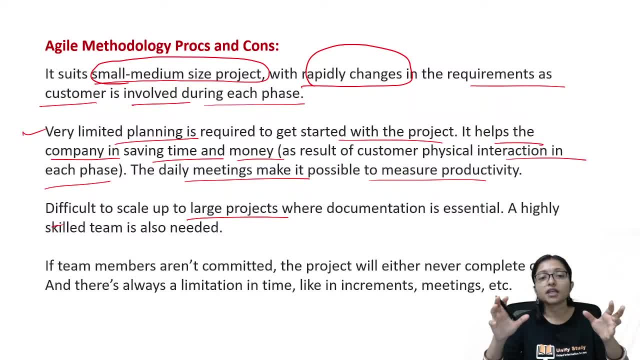 because in the large project that way it's not possible. for the large project, proper planning is required, proper documentation is required, as their we are not maintaining documentation. that's why for the large project- as i will be not good, okay, so highly skilled team also required for the large project. for this type of small project, okay, normal. 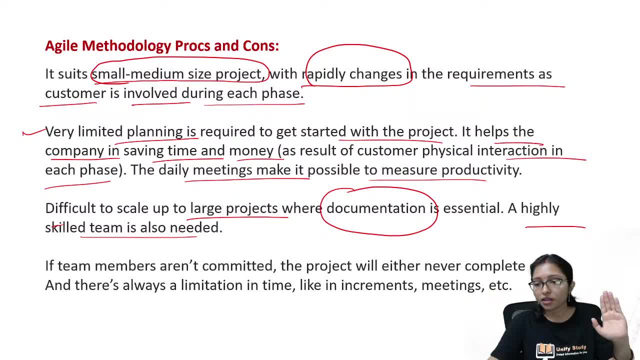 team will work. but for the what happened from my side to, there is no network problem. am i audible or not? i hope i. everything is fine right from my side. there is no problem. everything is clear, right, yes, yes. so if the team member are not committed, the project will never complete and fail. 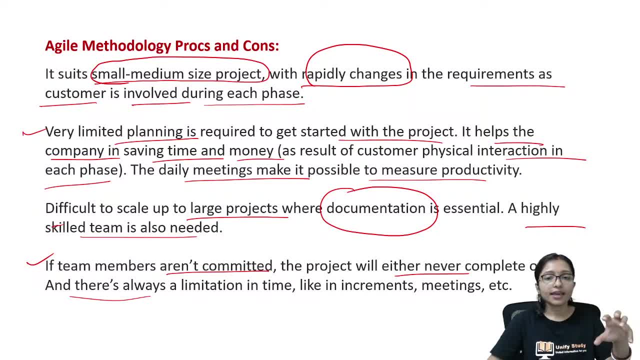 team member have to be committed. definitely, if team member are thinking, no, i will not do, then it will be not work, the meeting is not going to happen. so i hope you understand increment team member has to be committed here. then only it can be done. so these are the pros. 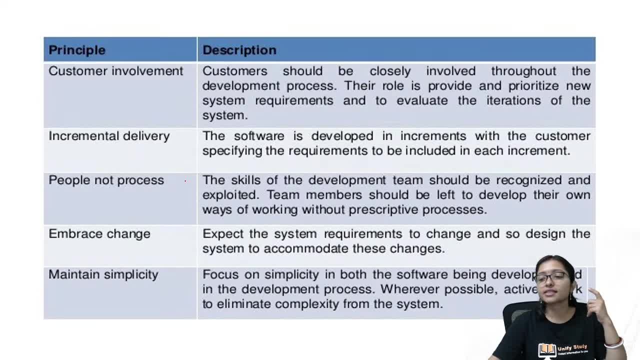 and crowns of the asile. and here you can see the principal. what are the principal main principal: customer involvement, incremental delivery, people, not process. very, very important. it is following on the people, not process, embrace change it embrace changes means any time any change can be happen. any time any change can be happen and that's why 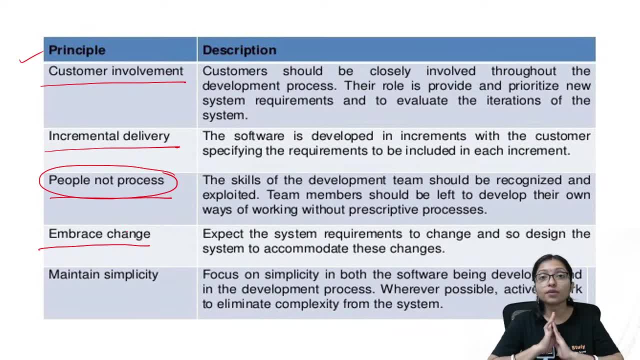 that's why the coding structure should be very good. proper framework, proper coding structure has to be there. if the coding structure is not good, if its proper framework is not maintained, then any time any changes cannot be done. just for example, if i am telling that key in the registration, now they are taking roll number, phone number and email. 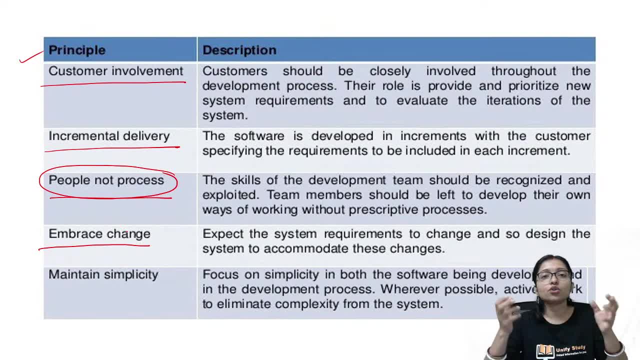 id. now i am telling that, no, i need to add an extra thing. okay, maybe some extra thing i need to add then. then that changes will be very much difficult to everywhere to show that. but if they are following the proper framework, then anytime any changes can be done. that is a. 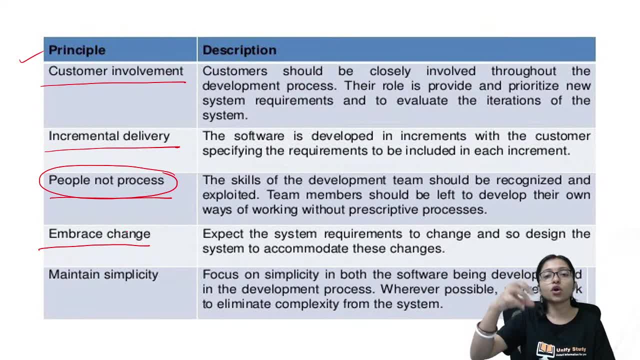 very important part and that's why coding structure will be also proper and the maintain the simplicity. as simple as that it should be. people, not process means: if you are following on the process, you have to follow this way, you have to follow this process, not like that. your team, your team members. 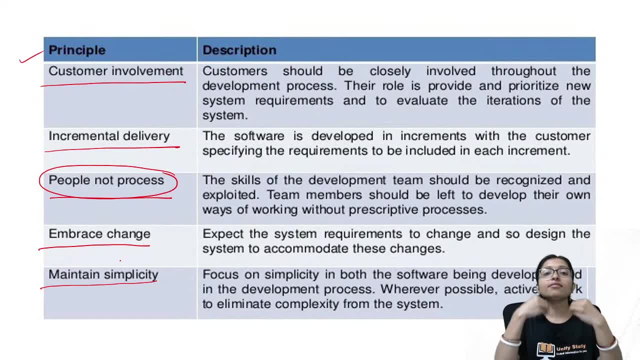 some, someone is there who is developing, leave it to them. yes, i am comfortable with this type of type, this type of way i am comfortable to write. okay, write it as per you, but ultimately my requirement should be done. if you are involving, if you are giving it proper thing, okay, this is. 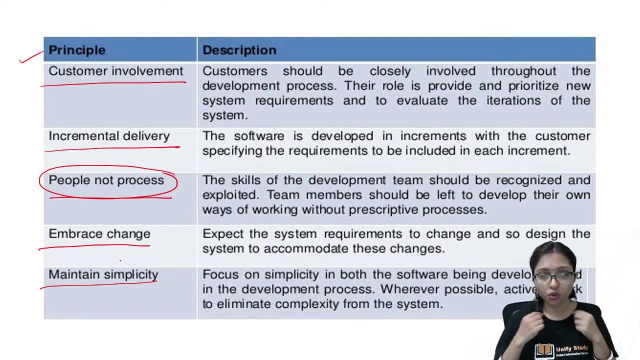 the process. you have to follow this way. you have to follow this process, not like that, your team process you have to follow, otherwise you cannot do. i am giving you that within this time. you have to do, you have to write the code like this way. so then there will be a fear, there will be some. 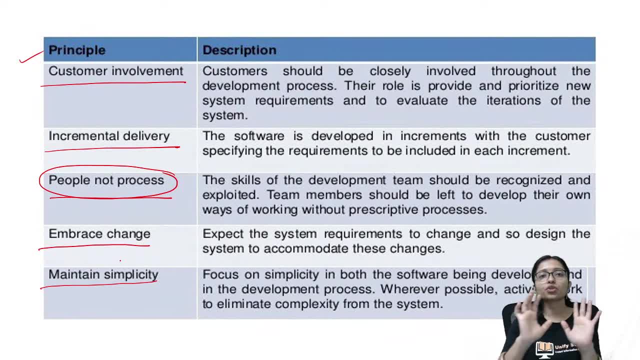 restriction and ultimately 100 output. they cannot give you. okay. if you are nurturing everyone as a friendly environment and if you are giving them independence, that as per do your best, put your 100 percent as per your knowledge, as per your creativity. how you are able to do it, do it. i am. 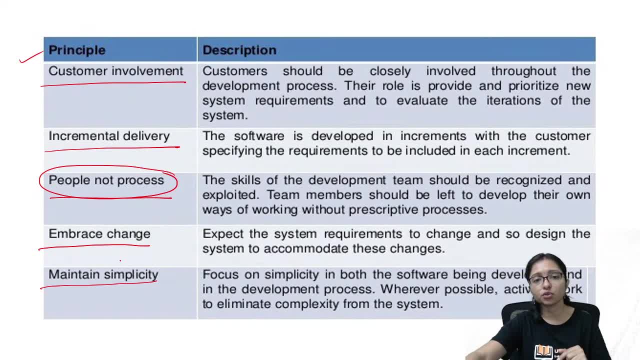 not giving any restriction, then your output will be good. that is called the people, not process. the skill of the development team should be recognized. who is good in this one? maybe one one of the team member is good in design, in good in javascript. do do them. yes, you can do it. so you can do it. 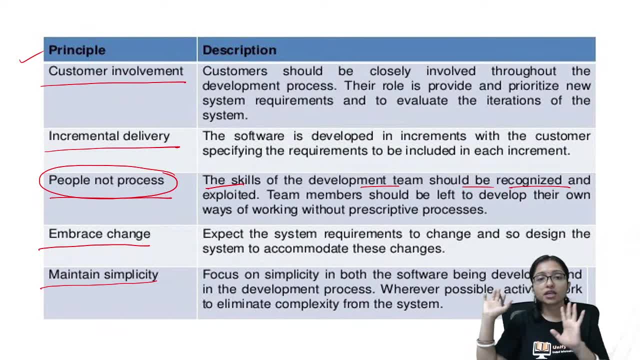 someone is good in dba database, tell them: okay, do it. let them choose, let them choose, they will choose. okay, i will do that. i will take that responsibility. you cannot force anyone that you have to do that. then your product will be good, got it. so team members should be left to develop. 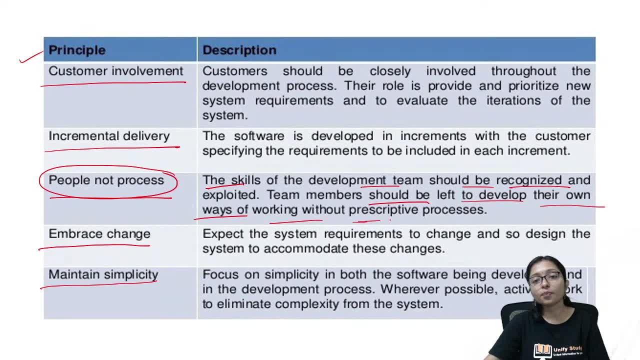 and their own way, working without perspective process. they will do as per their way. they let them do as per their comfort zone. don't force them. if you are forcing people with a process, if you are trying to bind with a process, then people will live like me, those people. 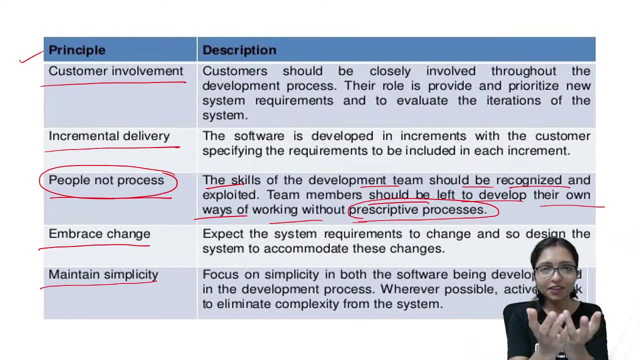 are like me. if someone is trying to bind with the process, rules and agreement, then like me, you cannot. you cannot bind me right, then like me, those people cannot do. like me. if you are forcing them will leave, anyone cannot bind them. that is the thing. if you are binding the people with a process, 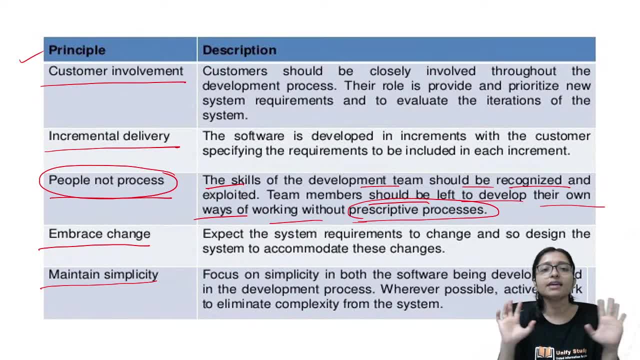 then definitely the good people will leave from your industry. they will be not there. it is, it will be, it will be there. so that's why you have to think about people, not the process. clear, is this clear? that is a very important part of as I incremental delivery so clear. I hope this all. 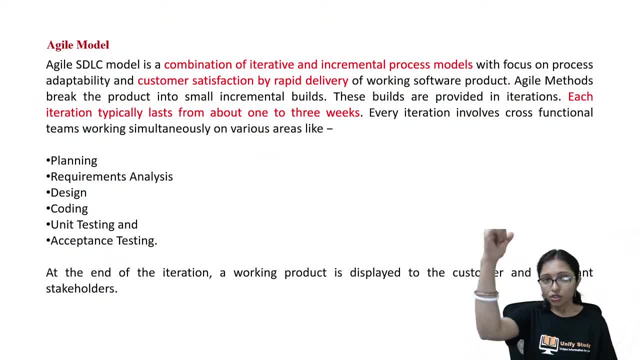 the points are clear to everyone. so right down what are the points of as a philosophy, main keyword, main keyword, ad use to come while watching live plus, if you can solve this issue, this is not a issue because the ad is giving you the some little bit money. the ads is giving you little bit money, well, while you are watching. 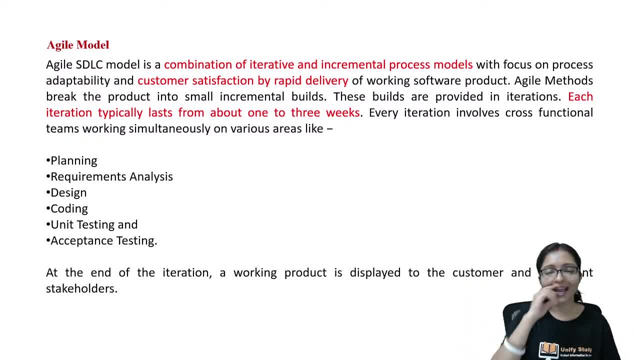 television, then also the uh, then also the ads are coming right. it's not very frequent. some time maybe just adjust it, because little bit money at the end of the day i also need, right. so if i stop everything, then from where i will get the money? very, very less. it's very less, but still. 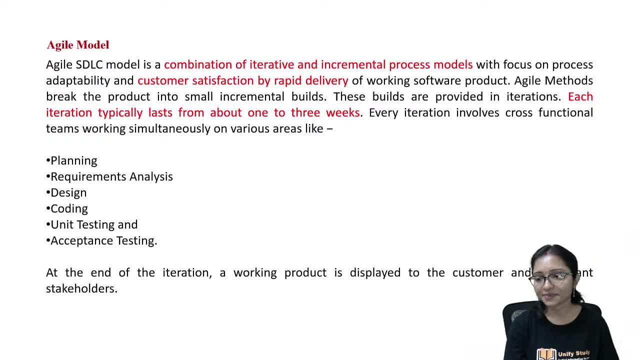 something for me also required. try to understand. okay, yes, tell me what are the main main concept of agile model? what are the main key feature? my question: what is your question? uh, parvati, what is your question? what is your question? can you please repeat? i am not able to see your question flexible. 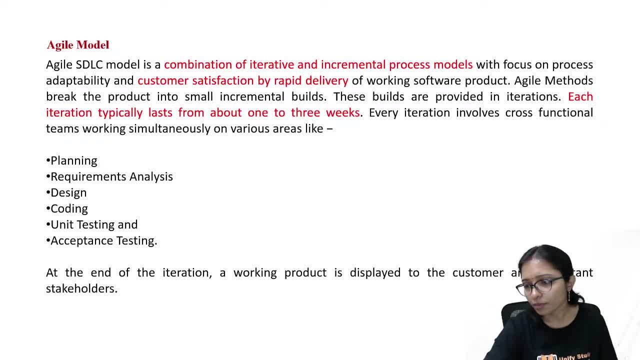 incremental delivery: people, not process. people, environment maintenance, embrace changes. customer involvement: very good. adopted new feature combination of incremental and iterative, flexible adaptive model. focus on customer suggestion rather than documentation. okay, good flexibility, customer involvement, rapid changes, small projects, long-term project means need hi ha very good. very good all of you. 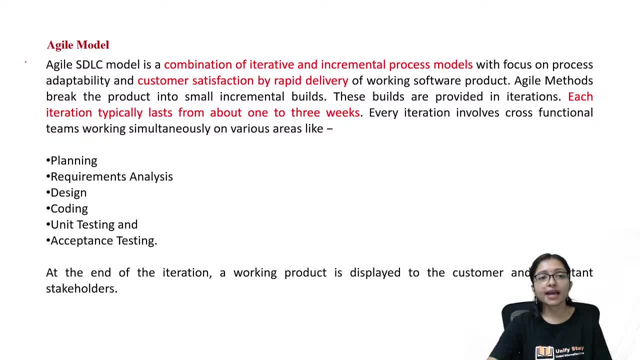 good. so here the agile model, as i sdlc model, is the combination of this. i already told customer satisfaction, rapid delivery is there and every iteration- sometimes questions are coming from here- each and every iteration will be about one to three weeks. it will be about one to three weeks, okay. 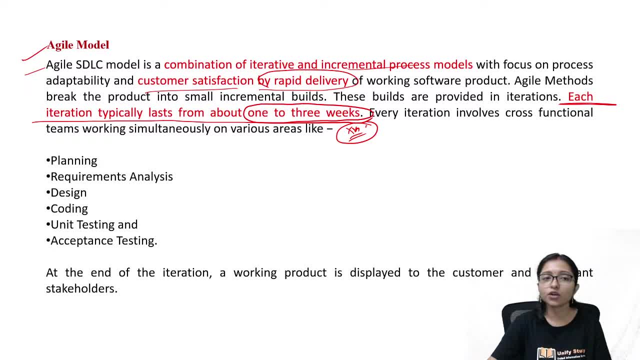 this is very important. each and every iteration will be one to three weeks, so every iteration involve cross functional team working simultaneously on various like the planning requirement, analysis, design, coding, unit testing, acceptance testing. okay, so these are the main concept and here the end of iteration is working with the display of the customer. yes, 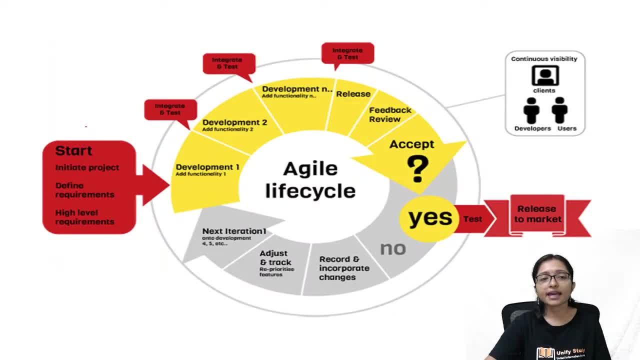 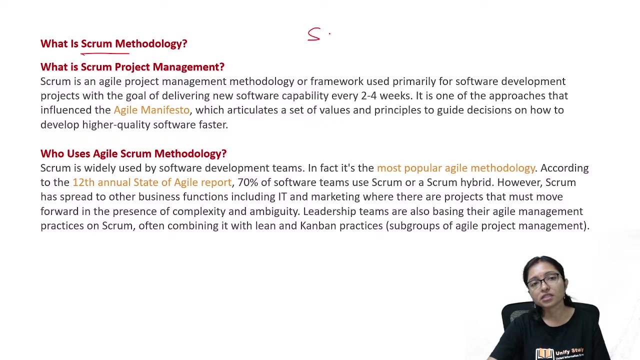 work tools, one through three, and then the end in Saro palms. its the logic of inner vegetation. this is the hard part 1, inner wat. you have to do the changes. then you have to do the changes right. yes, and here the scrum. what is scrum? scrum is that scrum is giving you the framework. scrum is actually agile is a concept. 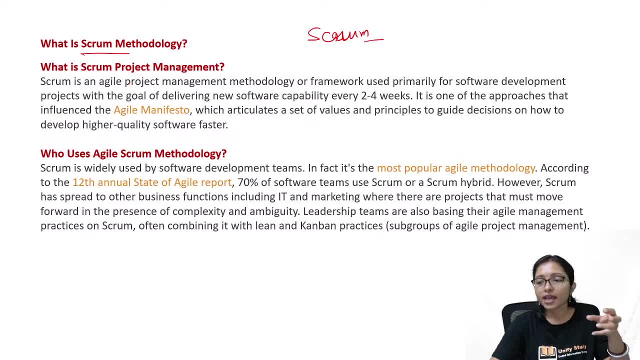 and scrum is the framework. agile is the concept, scrum is the framework. scrum is an agile project management methodology or framework used primarily for the software development project, with the goal of delivering the new capability within every two to four weeks. so this is a proper framework. through that framework we can implement the agile methodology. 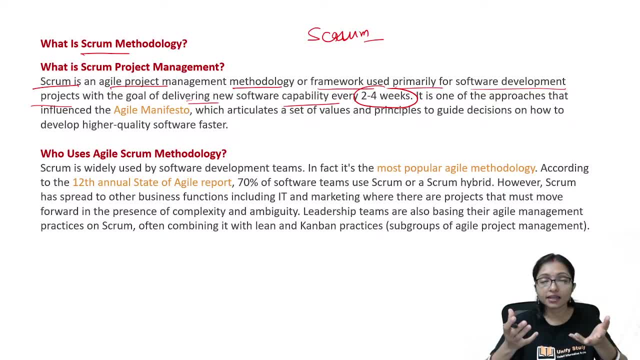 so that's why nowadays, scrum training, scrum master course, are very popular. if you are working in an IT sector, if you want to get the job in IT sector, then the scrum master training is required. means how to handle the team. how to handle the team. 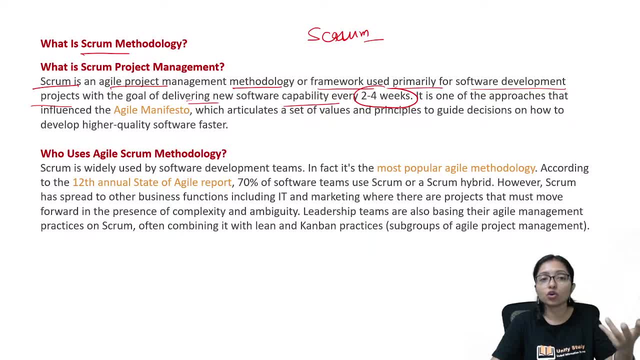 what are the framework we are going to follow. that is called the scrum. okay, so who use agile scrum methodology? scrum- most of the 70 percent of the software is agile scrum methodology. so who use agile scrum methodology? scrum- most of the 70 percent of the software is agile scrum methodology. 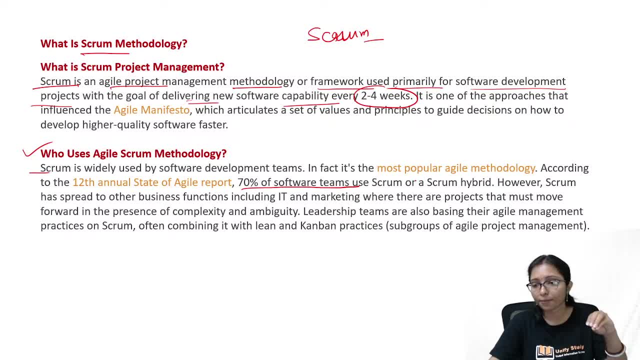 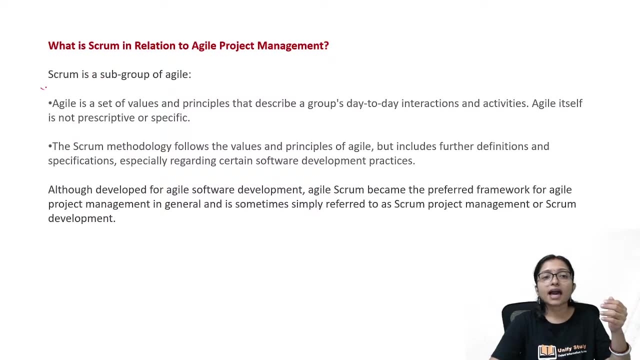 software development team are using that scrum. this is they are using. okay, so nowadays everyone is using that scrum methodology and IT marketing leadership team- all are using nowadays this scrum. so what is scrum? scrum is the subgroup of agile. agile is the set of values and principles that 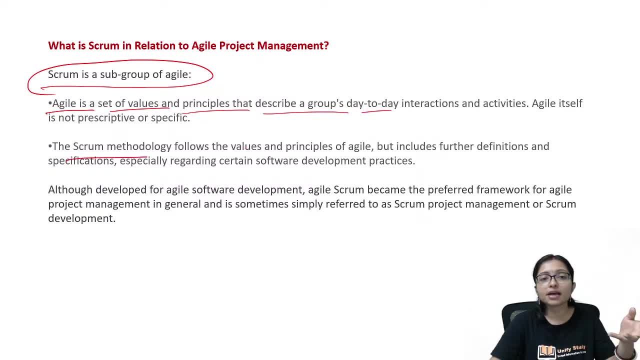 is a theoretical concept and scrum is the methodology. follow the values principle but include further definition, specification, how to follow that, how to follow that. that should be a proper framework. that is, that is scrum is giving you. although developed in agile sector software development, agile scrum becomes the preferred framework for the agile project management. 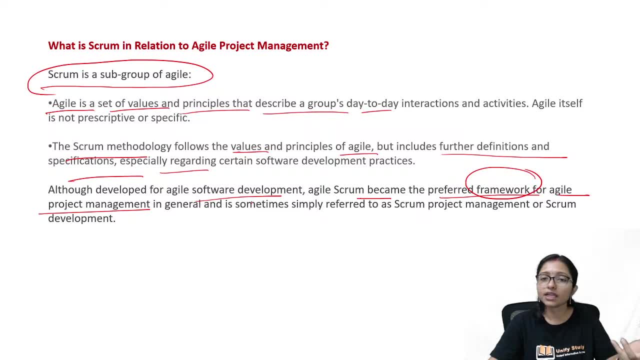 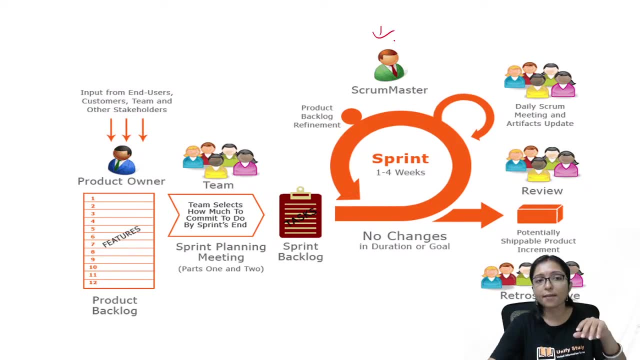 that is the preferred framework, got it. what is scrum? what is scrum? is this clear? you can see. it is a very clear example of scrum. this is the scrum master here. some concepts are there: product backlog- what is product backlog? product backlog means the feature list. I am the product owner. I. 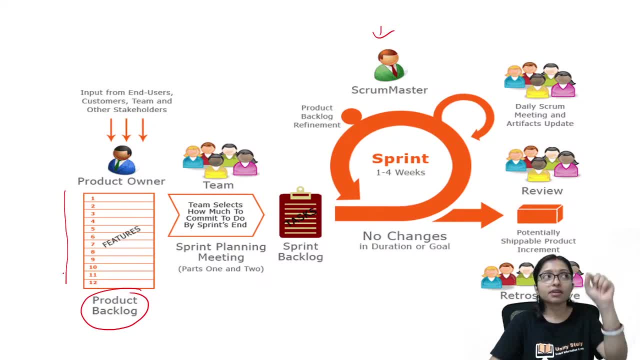 am the product owner of Unify study app, so I am giving the feature list. okay, so input from the user, customer and the stakeholder, that is the feature list. that is called product backlog, so log. now the team will decide. the developer team will decide that they will divide the feature. 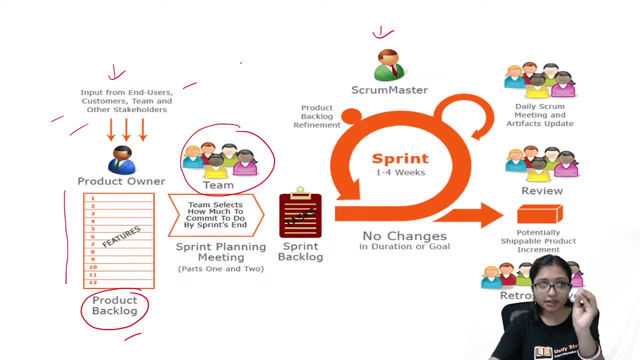 into some sprint. that is, within this print, very small time: one to two weeks or three weeks. within one to three weeks, what we are going to deliver, all the team member will discuss between they each other. it's not like that top down approach, it is a bottom-up approach. normal companies are. 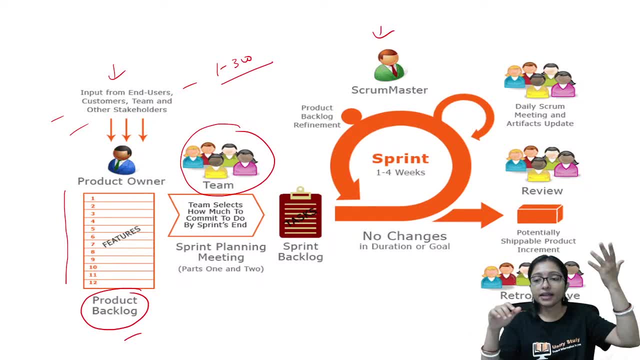 doing: company manager, company team leader, they will decide and they will force the team that you have to do it. but here it is a bottom-up approach. here total team are doing uh meeting and from that meeting they are taking that decision. okay, these are the things we can deliver. 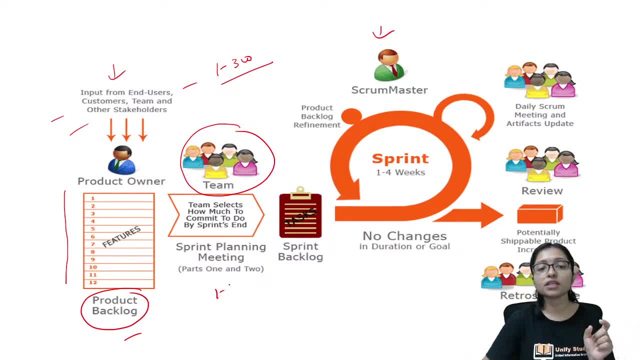 in this fast print. that is first. print means within this one to three weeks. we can deliver this feature. then they will write a sprint backlog. screen backlog means the first print, that is first. one to three weeks. we are going to deliver this. everyone will take the decision, not like that. 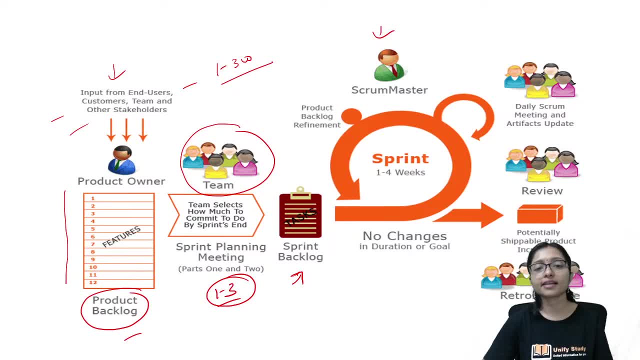 management will give that everyone together will take the decision and they will make the task list. after that they will start it. after that they will start it. no, here, they will start within four to within maximum one to four weeks. they will start, and every day in inside the development team also. 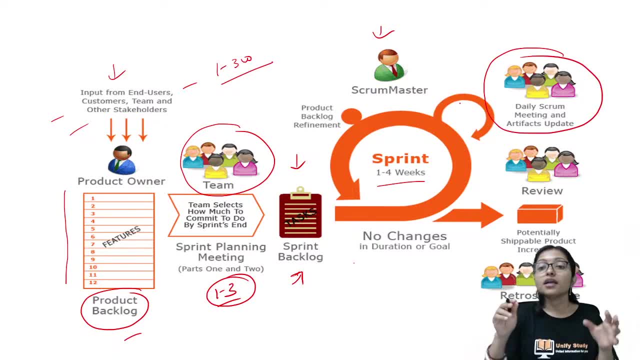 daily scrum meeting will be there. sometimes that is called stand-up meeting. in in companies they are telling the stand-up meeting every day. there will be 10 to 15 minutes stand-up meeting. everyone will be together and they will discuss that what is the situation of, what are the feature? everyone. 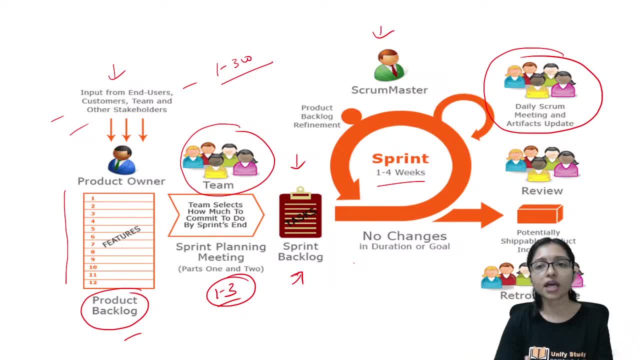 is doing and what are the update? everyone tell about the update. if they are facing some problem, they will discuss between the team member and after that they will try to resolve it. this is their internal process here. customer is not there in their daily scrum meeting. it will be happened. 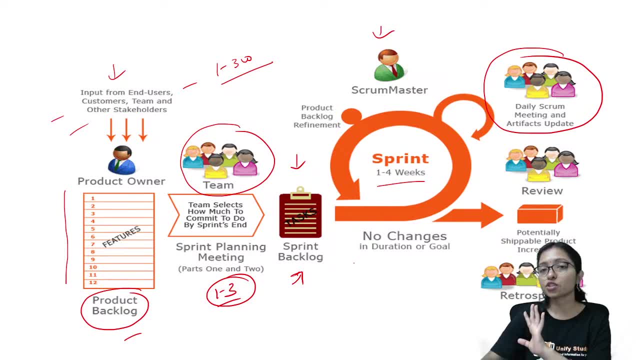 with the development team. their customer involvement is not there here. scrum master will manage that okay and they will review also the potentiality. also they will think that yes, we can do it or not, and after that if there is no problem, they will be able to deliver. that got it. this is the some. 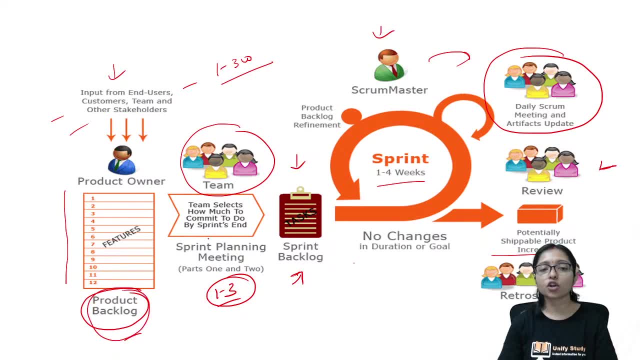 terminology. you have to remember what is product backlog, what is print backlog, what is called scrum master, what are the duty of the scrum master, what is the daily meeting, what is going on? so this is normally going on in companies and i hope it is clear to everyone. yes, this is clear to everyone. so here you can. 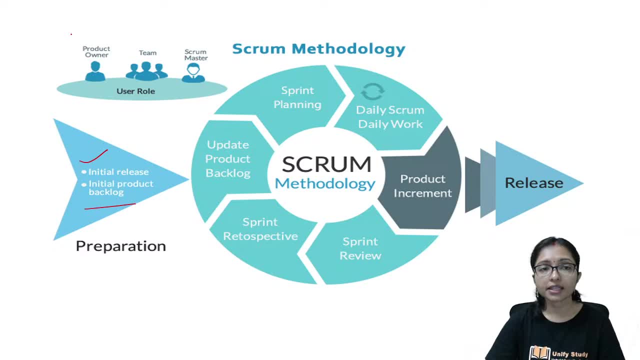 see initial release, initial product backlog. here there will be product owner team and scrum master. these are the different user role scrum methodology- you can see the scrum methodology is here: the update, the backlog, sprint planning, daily scrum and sprint retrospective and sprint retrospective review and finally, product increment and there will be the release. this is the process you are. 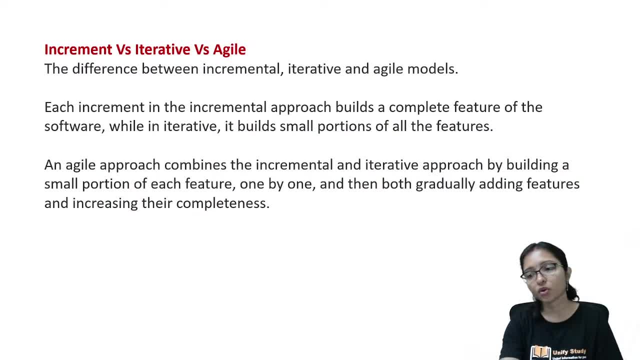 going to follow in agile methodology. okay, so here is the difference between agile, incremental and iterative. each incremental in incremental approach builds the complete feature, while iterative builds the small portion of all feature. and agile approach combine the incremental and iterative approach by building a small portion of each feature, one by one, then both. 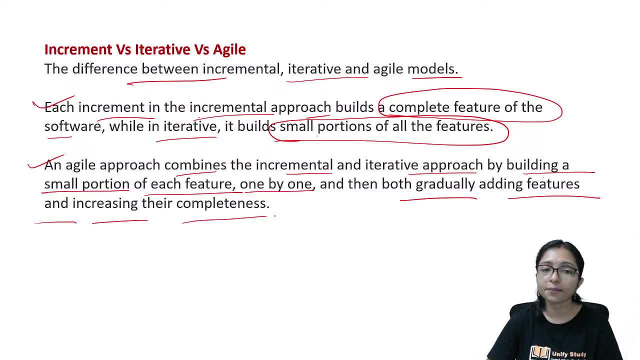 gradually adding feature and increasing the completeness- that is the main points- as much as possible using that feature, and then the other features are still mentioned. Now, ready, let us start increase way. i wrote here as much as possible. increase way so that you can understand the. 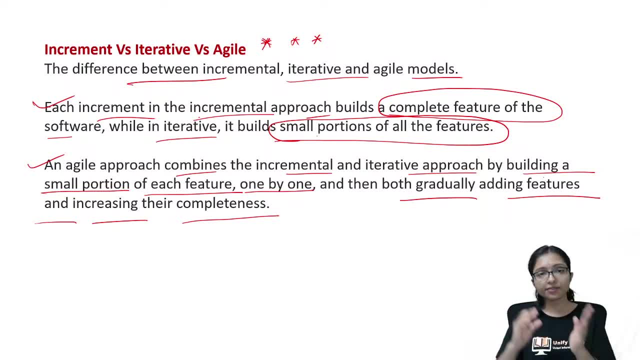 main difference between incremental, iterative and agile. is this clear? i hope with this line it will be clear. read it and tell me, is this clear or not? yes, there are hundred feature we have to do. incremental approach will do ten complete feature, then after that ten complete feature. that was the thing in iterative. it was like that. 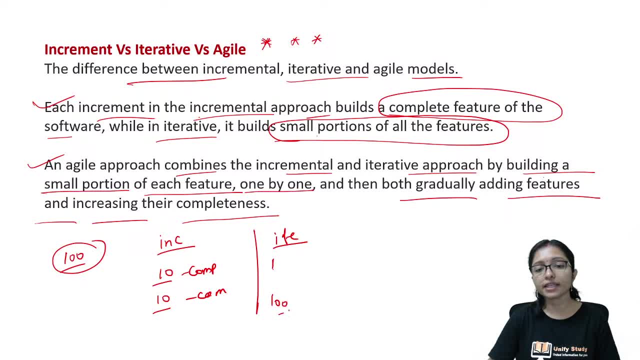 key: every hundred, one, two hundred, all they will do ten percent, ten percent like that, and here in agile they are doing. i will take ten feature out of then also i will do fifty percent of all feature. that is the agile. okay, clear, yes, yes, good, very good. 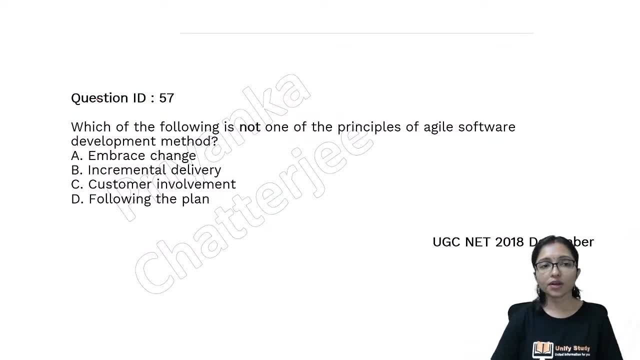 chalo, then do this one, then tell me what will be the answer of this question. what will be the answer of this question? what will be the answer of this question? this is the ugc net december 2018 question. ugc net- december 2018 question. 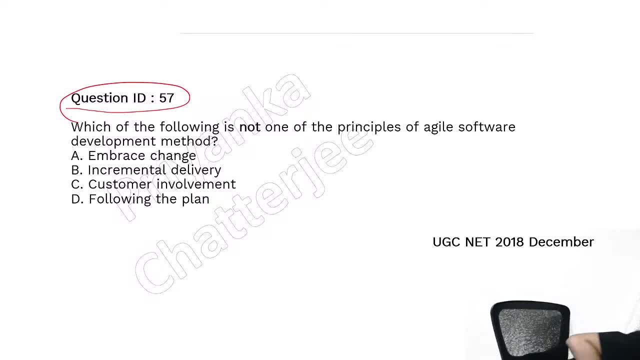 this is the ugc net december 2019 question. ugc net december 2020 question. okay, yes, that is very good. all of you are reading question very carefully. that's good. here, who is telling? who is telling khoda yaza, khoda yaza, take, uh and take, it is like that- and do ten. 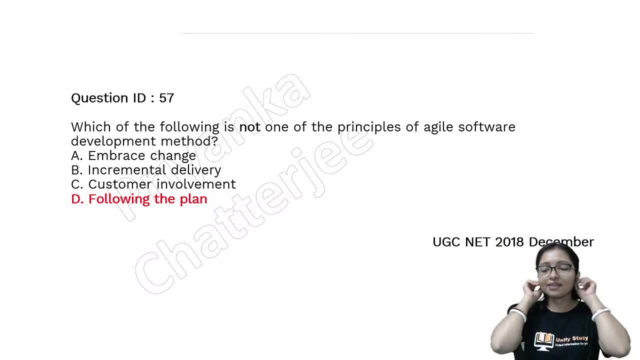 time. sit up, good as a. do 10 times it up. okay with your ears. do 10 times it up, okay. you are telling a here. it is asking you, not which one. is the, not what. i am telling that if you are missing the not, if you are not reading question properly, then you have to do not. qualified are you? are you? are you? 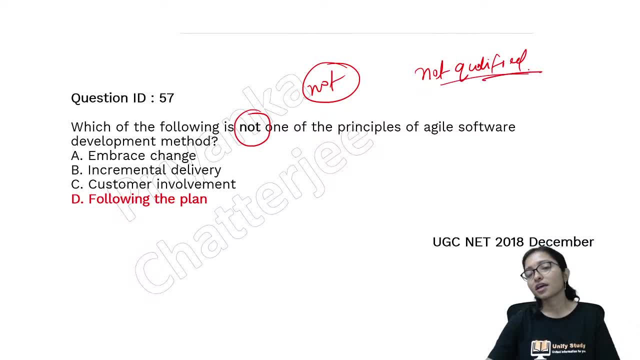 ready to see that? not qualified. are you ready to see that? only, as i did the mistake, i can see. money come also. money come also. you have to do 10 times. sit up, okay, and, and, and, and, so money come. and. khoda is it is. they are not not not one of the principalities also. 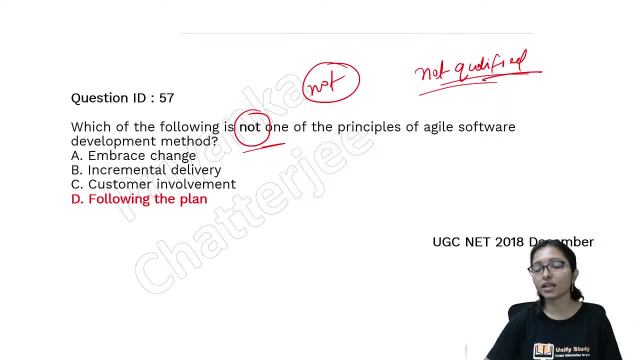 not, not. don't miss the knot. then you have have to see not qualified. then i have to see not qualified. be be careful about the not in the question. this is very, very important. you have to see the not. okay, very careful about that, very careful about that. 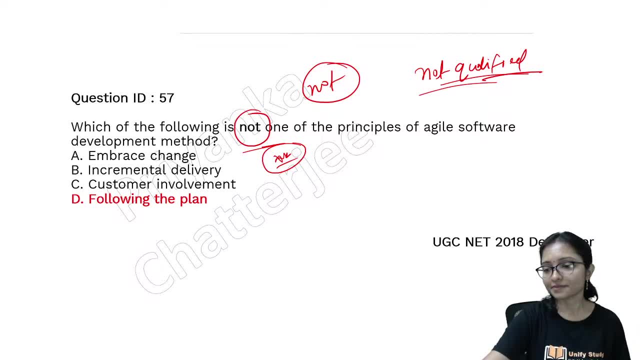 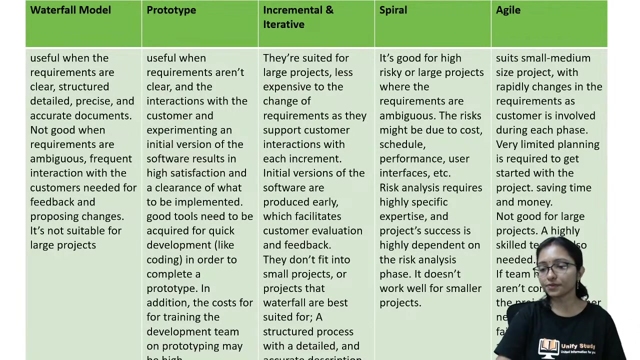 you. okay, is this clear? okay, okay, now do this. so here, this is your now. here, this is your different types of model. you can see, this is the different types of model. this is your quick revision note. this is your quick revision note. waterfall model, prototype model. incremental model, spiral model. 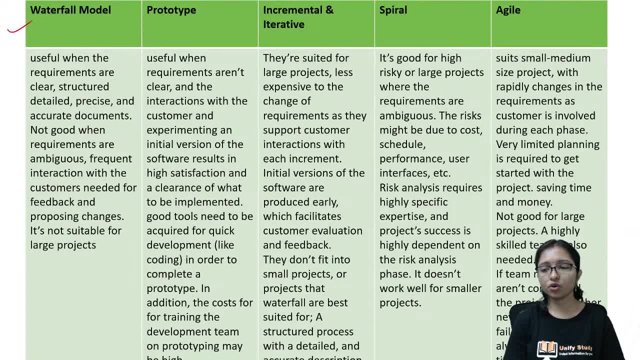 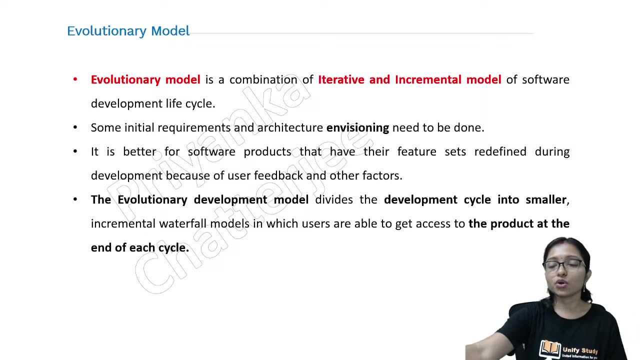 agile model. this is your quick revision note. you can go through this quick revision note for your exam. okay, for your exam, and that is the. that is the things you have to do. okay, clear, clear to everyone. yes, yes, yes, so chalo. so here, now we will do. i, i will upload this in app. i will upload the pdf. 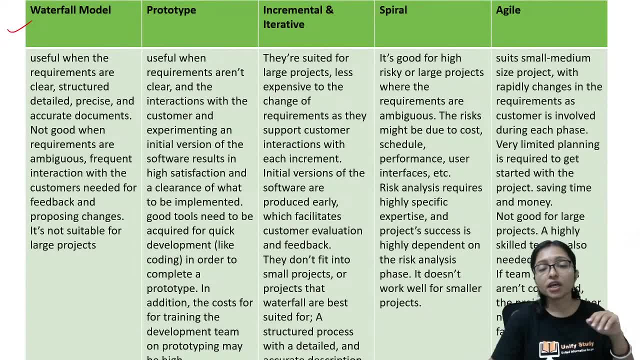 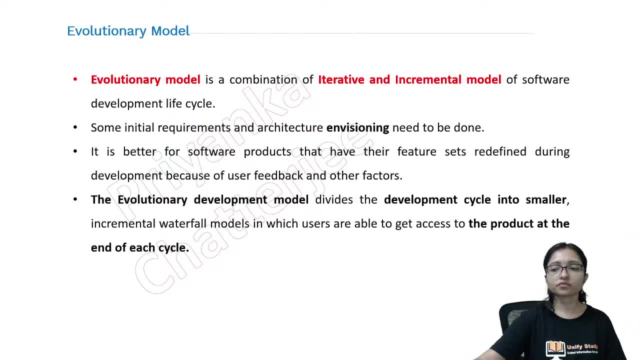 pdf. pdf of the sdlc model, complete pdf. i will upload in unify study app. all of you, you in the study material section, you will get that pdf. okay, the sdlc model pdf, free, i will provide, you can, you can download it and you can check it. okay, so here here what it is: evolutionary model: what is? 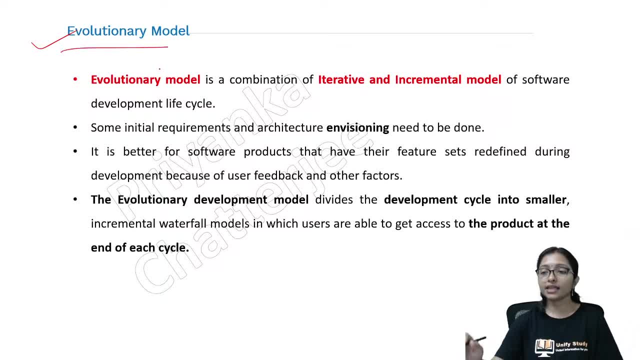 evolutionary model. here the evolutionary model is the combination of iterative and incremental model. okay, evolutionary prototype is different and here evolutionary model is also there. some initial requirement and the architecture is here. that is what evolutionary development model divided the development life cycle into smaller increment. waterfall model is used. the 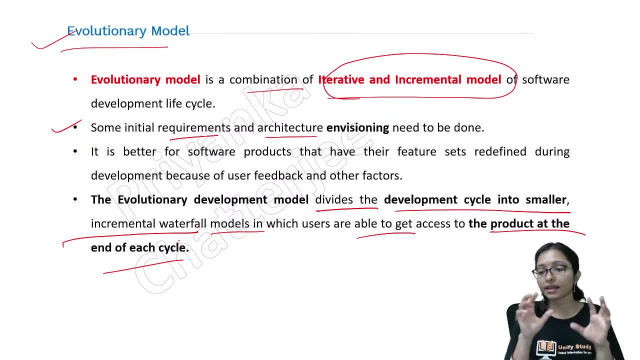 user for the product at the life cycle. so the smaller here it's here. here it is the smaller part you are dividing. each and every one is divided into the smaller part. that is. that is most important part, okay, okay. so for laptop, i will provide the link we are integrating for laptop very soon. you. 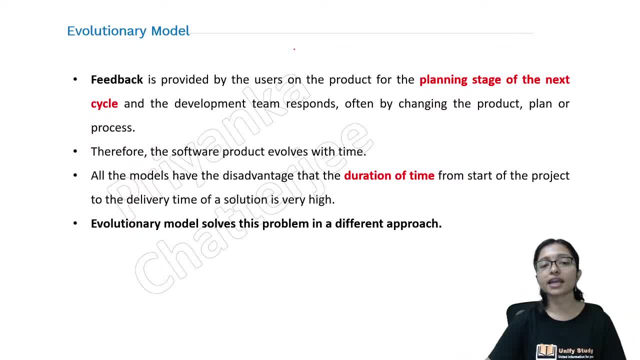 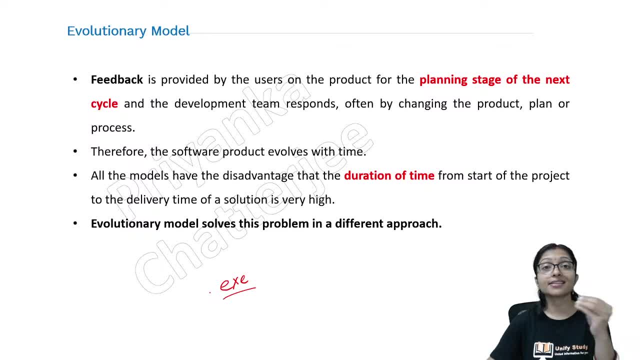 worry about that. it will show you some alert like that it risky and all. because whenever you are installing any exe file it will show you alert. but i will do the checking and after that only i will share, you don't worry about that. so if you are installing that exe, then you can get the desktop. 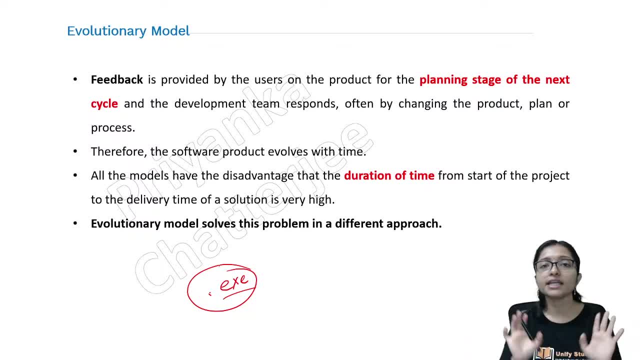 version. so in the desktop version you can get the desktop version. so in the desktop version you can version, you can open it in your laptop or in your computer. and for website version also very soon i will provide you the website version also very soon within, i hope, within one to two days i will. 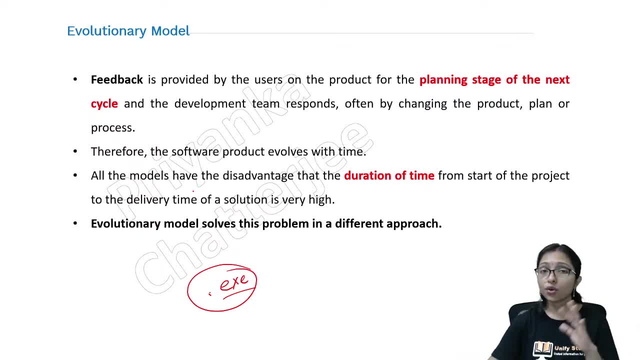 provide you maybe next week. within next week you will get the website version also. i will provide you the website version so that you can read it in in your laptop. okay, okay, print out. for that i have some restriction. till now i am not giving anything for print out. latter we can think about. 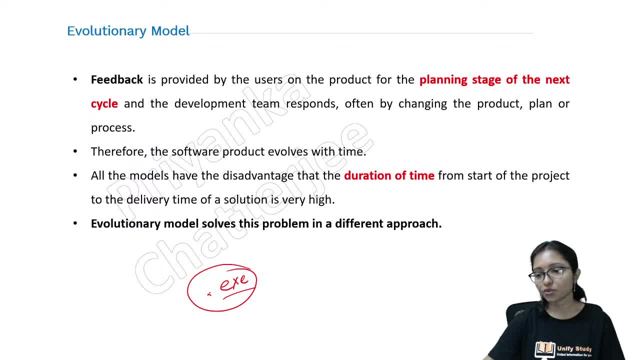 print out. till now i am not giving anything for print out, okay, okay. so here, feedback, here the feedback, feedback of the user planning stage in the next cycle. feedback is the important here and therefore software product involving time: okay, website, i will, i will, i will go, i will give you that website. so, all the all the model disadvantage about the 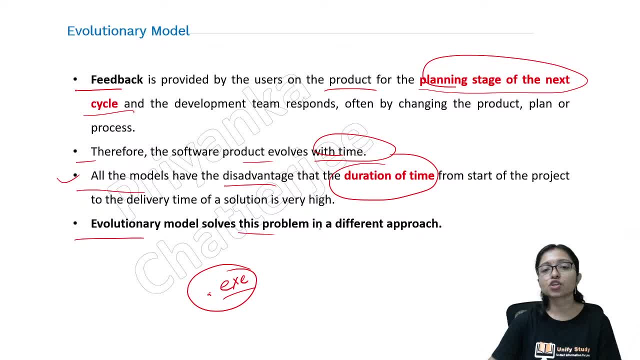 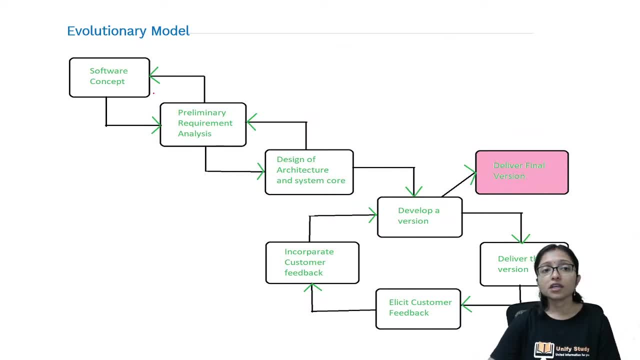 duration of time. okay, so evolutionary model solve the problem of different approach. here you can see the evolutionary model: that software, software concept, preliminary requirement analysis, then design of the architecture of the code, then develop a version one by one. we are giving the version in compar and then develop, delivery, the final version. so 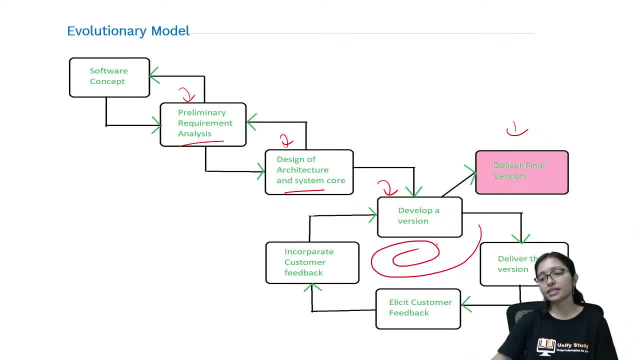 one by one, the version will be done and it will be said: that is, that is the evolutionary model. only, just, a, just just. we are dividing into small, small part. okay, so here you can see: initial raft requirement, then specific format. ok, there is final requirement, the finally are completed and out there. also, we come to this: 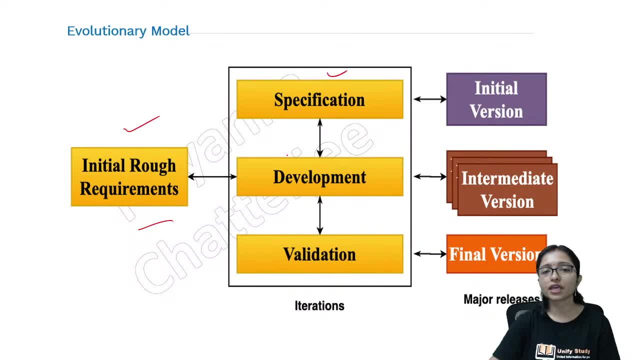 uh, get thebook Mutta author to rest therapies or any other discussion about the final user model. then develop an intel vision. we will have a review on and about this as a result. requirement then specification here, initial version, then development, intermediate version, then final version, just like incremental, just like intimate iteration and incremental, uh same. 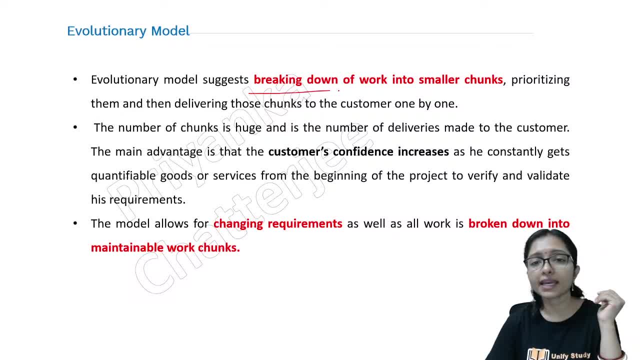 same way. okay, so main concept is breaking down the work into smaller chunk and then deliver the chunk to the customer one by one. number of chunk will be huge and that's why customer confident will be increased if you are giving small, small part and model allow the changing requirements also, as well as broken down into maintainable work chunk. so main concept: 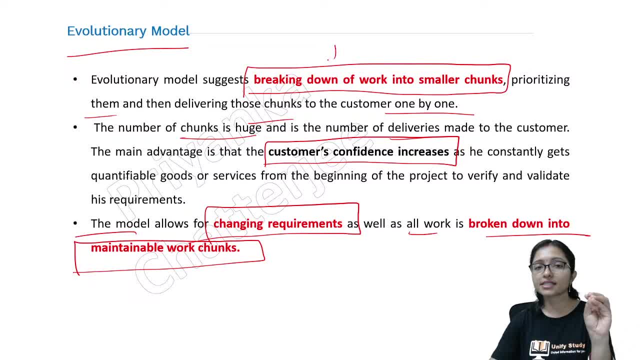 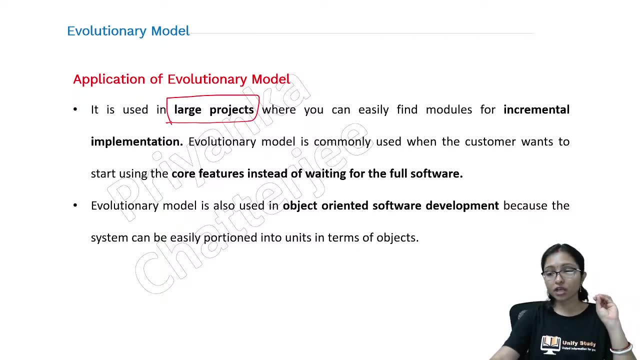 of the main keyword of the evolutionary model is the breaking down everything into smaller chunk. that is the main concept of evolution. this is the main keyword you can remember. okay, so here, whenever it is a large project, because see that agile methodology you cannot apply for the large. 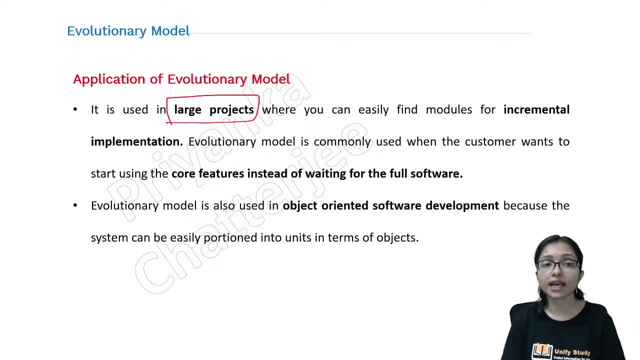 project, then for large project, what methodology we can use? for the large project we can use this evolutionary model. the large project we can easily divide into small chunk in some incremental incrementation, and then we can deliver. that is the main concept of evolutionary model. agile is not able to do the large project right. that's why it is required the evolutionary model. 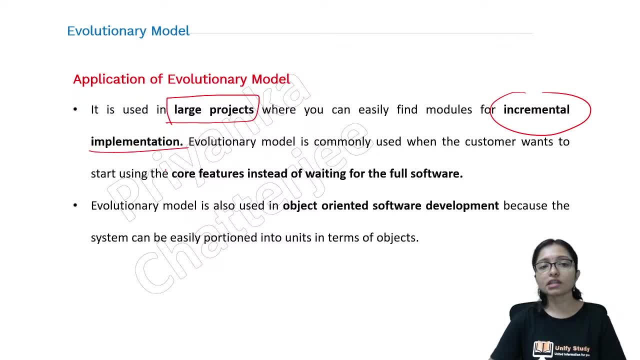 so it's incremental implementation and once start during that core feature, instead of waiting the full software. okay, so here, object oriented software development based on the system. here you can provide the object oriented software development. evolutionary software development model is also used for object oriented software development because the system is easily you can. 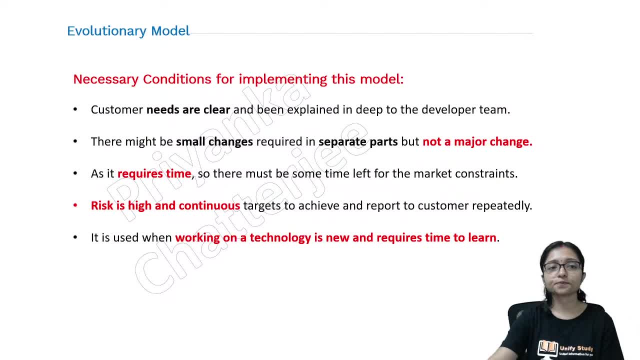 integrate here, okay, okay, clear, when it is necessary, necessary condition, when customer need, needs are clear, then only you can do as i leave. cannot do here as i. when it is not clear, then also you can start completely. okay, what is your, what is your doubt? parvati, what is your doubt? 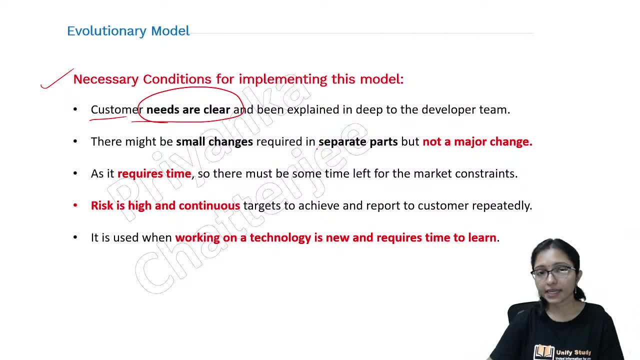 what is your doubt, parvati? tell me yes. so here the small changes separate into part, not a major change, as requirement time is there and market constraints are there. risk is the high and continuous target of the customer repeatedly and working on. the technology is there, but the best option is when you want to do the time the same time and then you will. 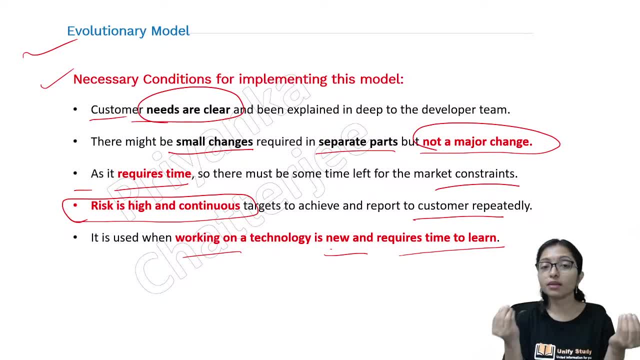 start able to do both: evaluation model in the case of döntar wykon model, stepwise leading to новых, merge of the terminology and choreography, osatsu dragei, time planning technology, new requirement to learn, new whenever the working on the technology is new and it also need time, it is also need time, okay, new whenever the priority, when the working on the technology is a new and request time, then it can. the time, then it can be also this at the main concept. evaluationary model. why i am telling question already came from here. this is also an important model. the evaluation type and evaluation, or maybe you will be confused. so it is a common step: evaluation or changer, insight technology, meta resulti of iterative version, and one- and you also learn that idea krenschert has a different function in lised, settled, deceived. only we will especially rizhasle social business, such as similar personalization of our premise of these terms. that is why ev cooks the work셨� mainly followed. 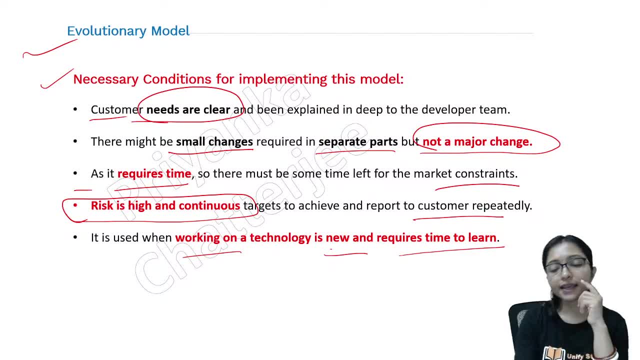 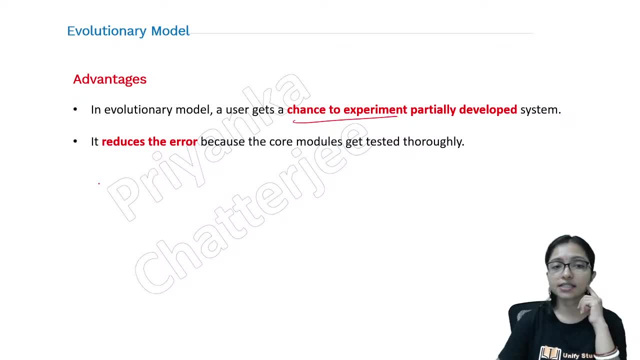 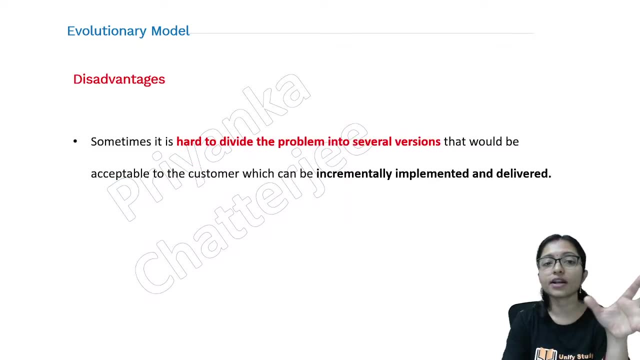 of iterative and increment. ok. so advantages are there. you can see the experiment partially. development chances reduce the error because of the core module. get tested thoroughly. that is the advantage. disadvantage: hard to divide the problem. that is very hard. part. what part i will do, what part i will not do? how to divide the everything? that is a very hectic task and incrementally. 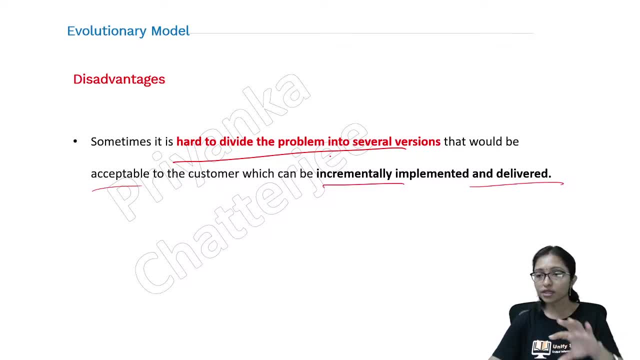 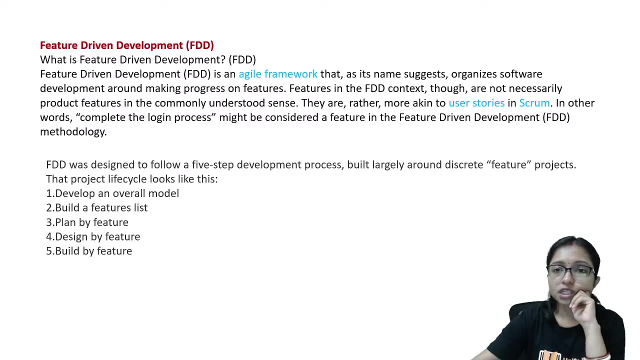 implemented and delivered. it is acceptable of the customer. this is little bit disadvantage. otherwise it's ok. clear- is this clear? evolutionary model: is this clear? next one is the feature devend model. feature devend means you are dividing prototype model. spiral model. development 3 comes under evolutionary process model. 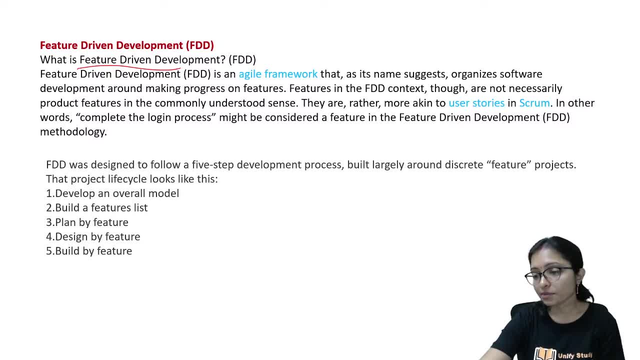 okay, no, no, no, no. prototype spiral: concurrent development model. this 3 comes under evolution. no, evolutionary process model. it is evolutionary model, is a different model. it's not coming under. it's not coming under this model. it is a different model. it is a different model itself. okay, it's not coming under. see that every time we are, we are. 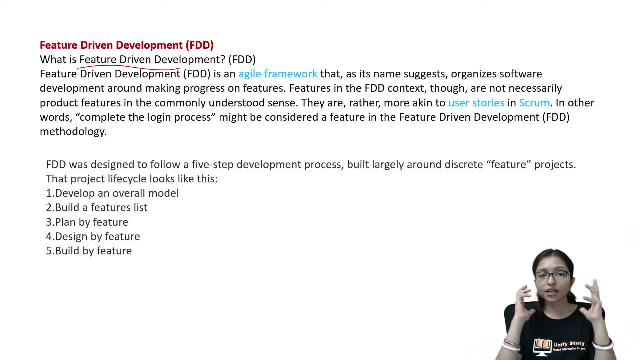 increasing the advantage. okay, every time we are trying to add something more, some concept from waterfall, some concept from prototype, some concept from iterative- we are combining them together and we are making another one like that. so feature driven model means it is dividing feature wise. one feature, second feature, third feature, feature wise: it will be divided. that's why it is called. 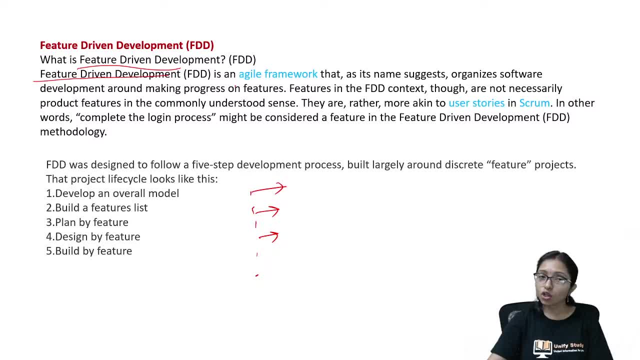 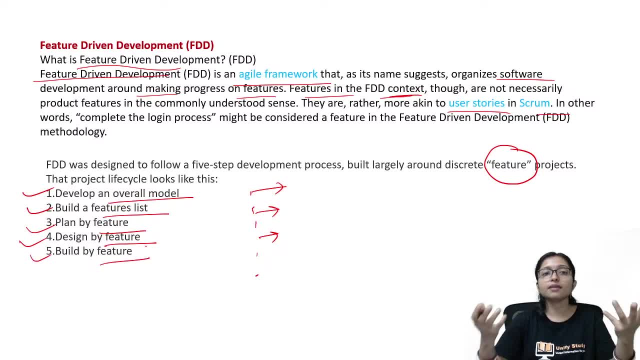 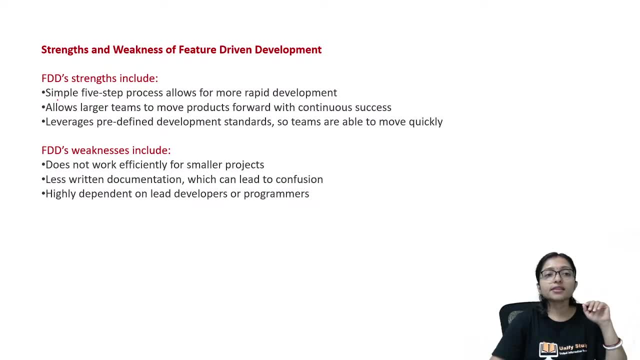 Developed by the feature. That's why the name is feature development, Feature driven development. Okay, Here the strength, Simple 5 steps are there, So we will do here for more rapidly development. Allow the large team to move the product Continuously because, feature wise, everyone can work And it is predefined development. 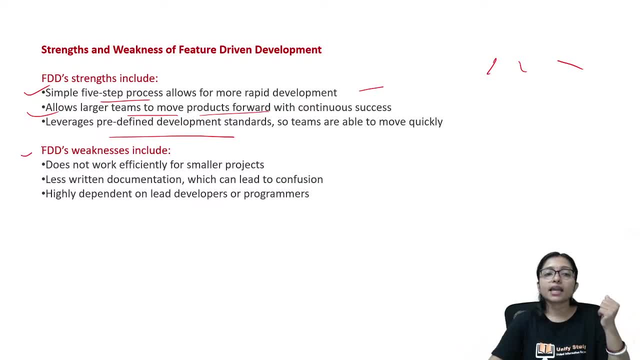 So more quickly team can do it. But FDD weakness are Does not work efficiently for the smaller project Here. these are working for the big project Because in the big project only you can separate a feature. This feature we are going to do When a feature itself will take maybe 1 month. 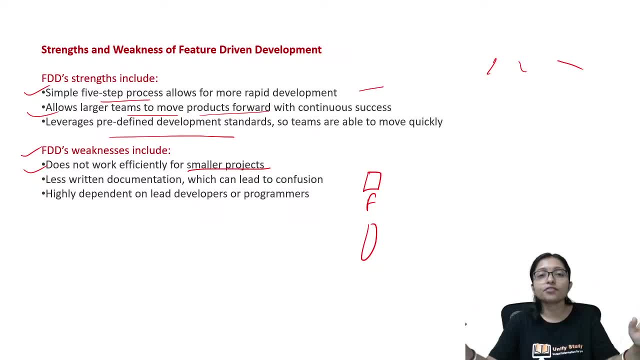 In a small project, you cannot divide the feature. In a big project, only, you can Divide it. So for the big project, you can choose this type. Less retain documentation, as it is following agile, So documentation will be not there And highly dependent on the lead of the developer. 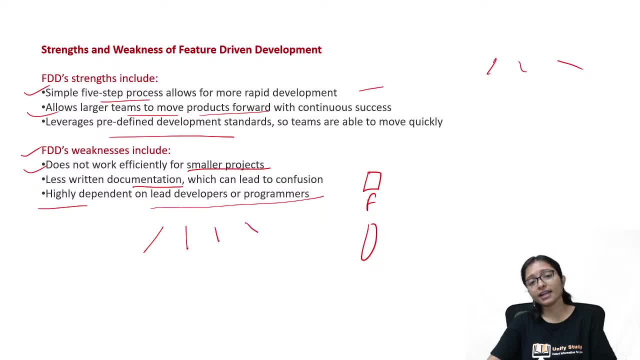 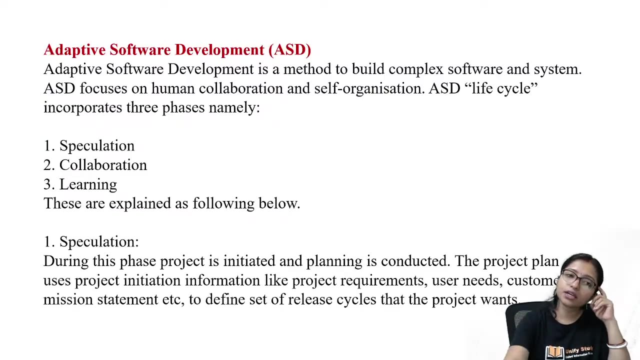 Because lead of the developer is only dividing the feature And according to that planning only it will go. If the lead of the developer is not that much strong, Then it will go. That is the Main disadvantages of feature driven development. Another one is adaptive software development. That was already. we saw one type of adaptive software development. 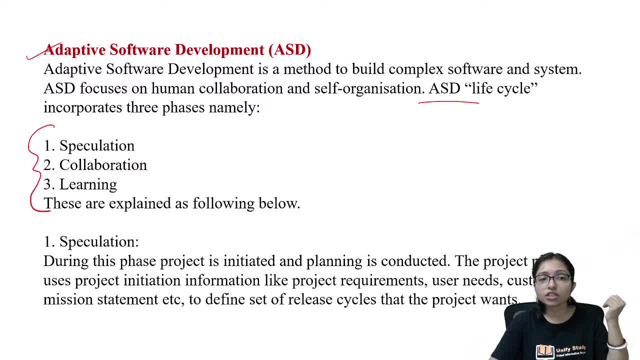 That is called ADS Here. these three terminologies are very, very important. Question came already from here also: Speculation, collaboration and learning, These are the three phases of adaptive software development. Speculation means during this phase project Initiated, the planning When the actually requirement initiation is going on. 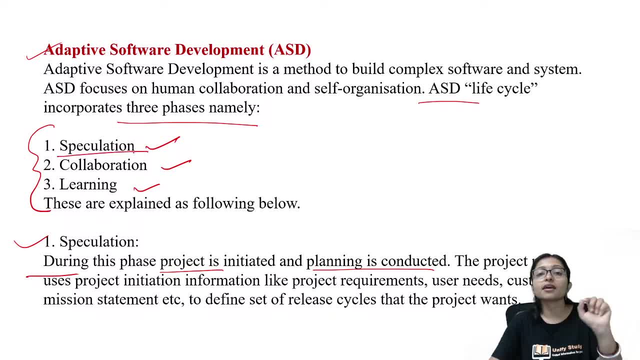 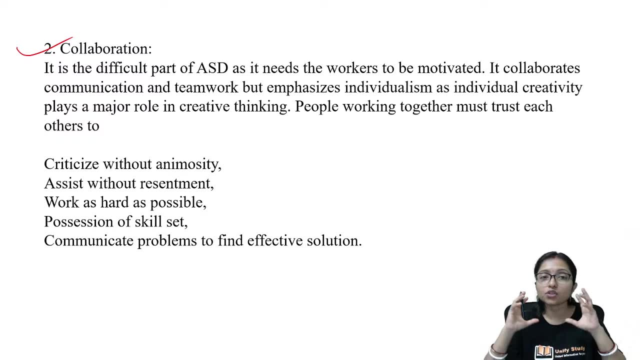 That is the name, speculation. Only they rename that as speculation. The planning phase. This is the planning phase. Next one is the collaboration, Where everyone collaboratively work. All the team member is working collaboratively. So it is the most difficult part of ADS Speculation is the spelling planning. 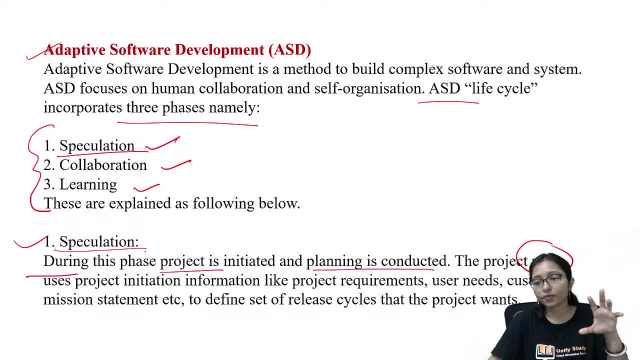 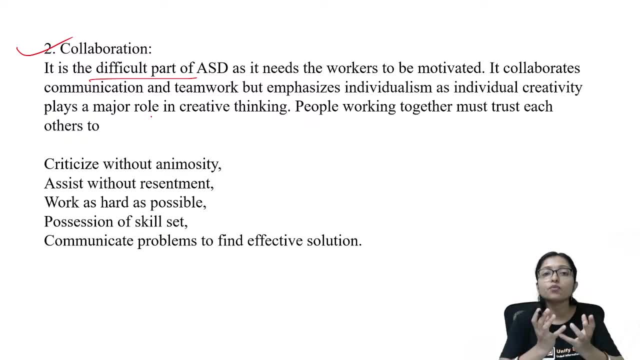 Speculation means that is the planning part, Okay. Next one is collaboration. Collaboration means here, Where every team member are working, So teamwork done. Emphasize the individual creativity, They will give the individual creativity, But collaboratively they will learn work. That is the part of ADS, The most difficult part. 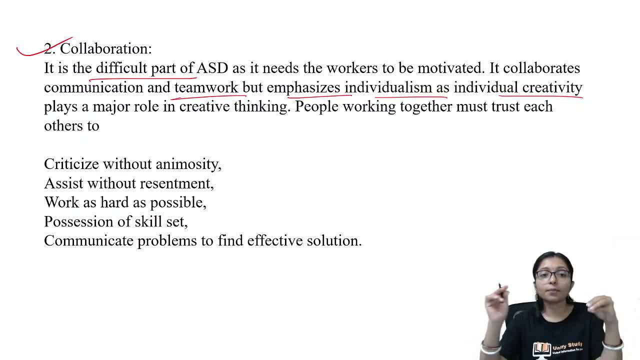 Everyone is itself doing their creativity, But it's together, People working together, and must trust each other. Criticize without animosity. Means- criticize will be there, But enemy type behavior will be not there. Assist without means: if you are, You can assist them, But if you are not telling them, 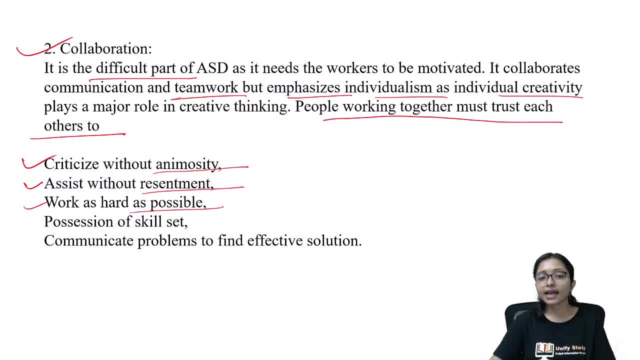 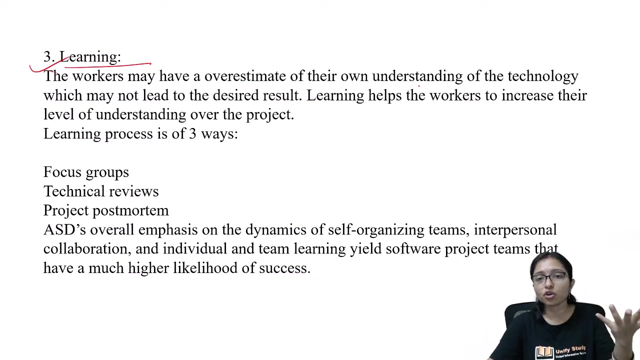 Some negative thing: Work hard as possible. Possession to the skill set, Where skill set is very important. Communicate problem, find effective solution. This is focusing on the team behavior. Team behavior is very, very important here. Learning is also important, As they are working on new technology. Understanding new technology is also important. These are very important factors because they are working on certain things, But you have to understand that It's not the other way around. It's only on two things: You have to work together and hopefully you will succeed If you are not satisfied and you can work together. 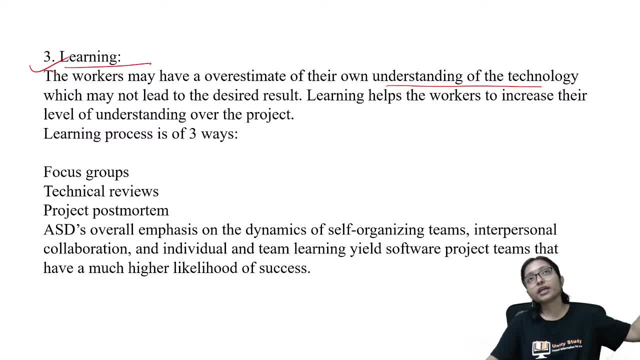 With them and your team members. So advanced model, waterfall model- those model was old model. These are the new model, where always team member has to be ready to learn new things. That is the learning part is there. So learning process three ways: focus on group technical reviews, project post term and means there will be training technically. there everyone will help and after that maybe some requirement will be there. then you have to learn by individually also. 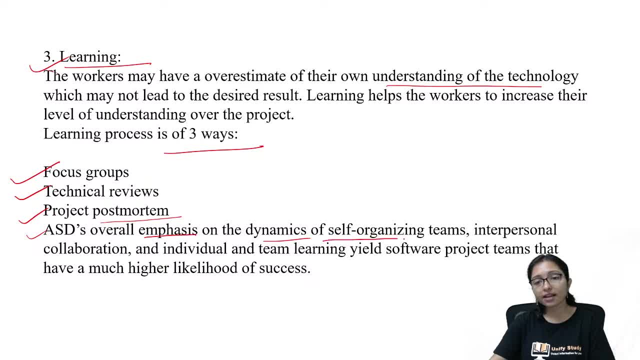 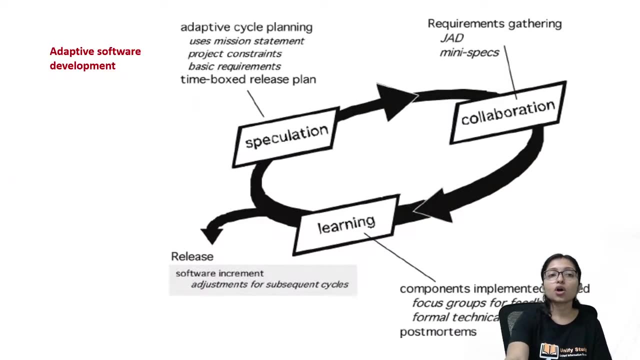 Overall emphasize on the dynamic of the self organizing team and interpersonal collaboration, individual and the team. learning will be also. This is the focus, main, key word- definitely remember- of adaptive software. you can see the speculation: collaboration and learning. These three words are very, very important. question already came from here. I am telling you: 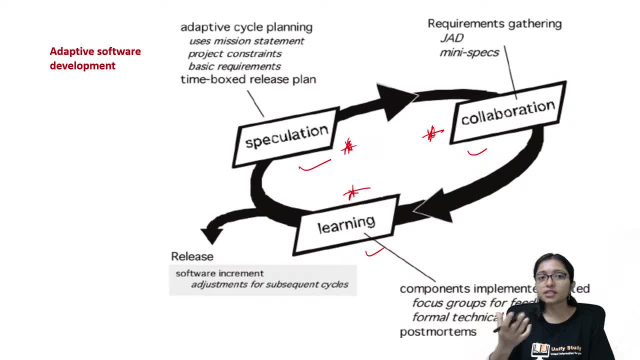 Maybe most of the area, most of the sources. you will not get this. you are not going to get this adaptive development and all others. these are important. Okay, yes, tomorrow also I will take the class. I promise myself upcoming all the day. I will take the class because I missed a lot when I was not able to upload content here. I was restricted, that I cannot upload any video, I cannot do anything in YouTube. it was pathetic for me. and when I am free now, I am independent now. 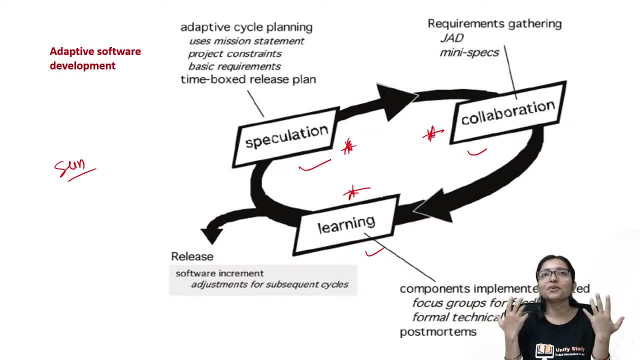 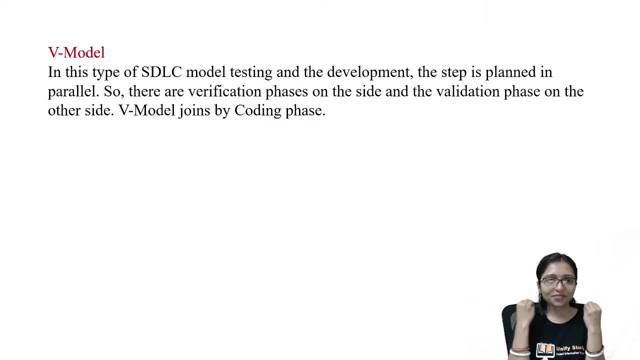 Now, Now, Now I am feeling that I have to. I want to do something. really, I missed a lot. that's why Sunday also, I will take the class. Sunday also, I will take the class I missed a lot. it is a different feeling. I feel that everything is nothing, nothing. it's nothing for a dream. it's nothing whenever we have a dream and if anyone is restricting you that you cannot do anything. 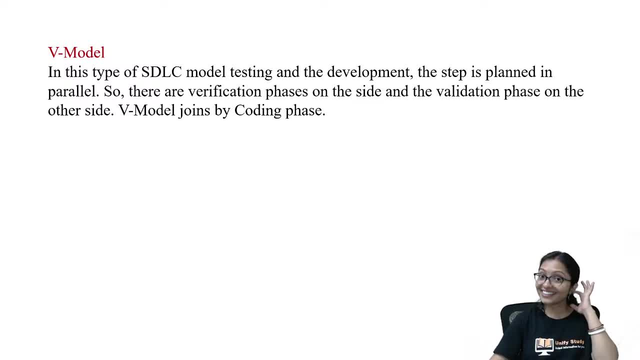 Then, then it is very pathetic. so I will take the class on Sunday. I will take the class we model. here is the we model. what about paper one? paper one, something interesting is coming, paper one, I hope Sunday. Sunday we are going to announce the paper one. good course, some good, some surprise is coming. 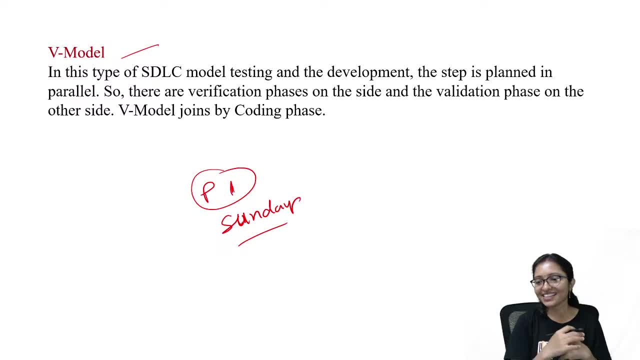 Coming for you for paper one one. surprise you surprise that coming one, surprise that coming for paper one. I hope Sunday we can give you the surprise. I hope Sunday for paper one I can give you the surprise. okay, okay, yes, And And And And paper timing will be same Sunday also, timing will be same. yes, timing will be same. for last one month I was thinking that I am in a jail. really, I was in a virtual jail. I was thinking I was in a virtual jail, I cannot do anything. 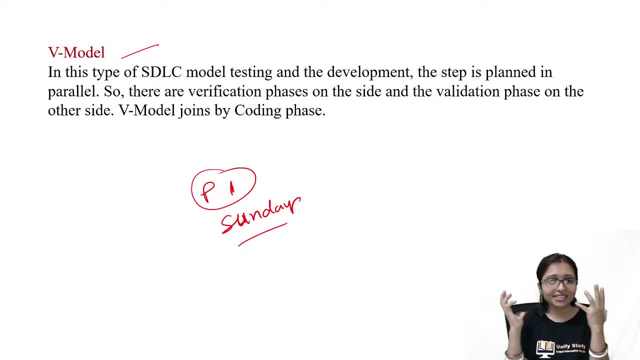 I cannot do anything. I am not at all free. I was restricted with the rules and that was a jail for me, so it I was not able to tolerate at all that jail. oh my god, it's not possible. it's not possible. so there may be money- money is important maybe, but it's not possible, right? yes, so we model. what is we model? we model, joined by 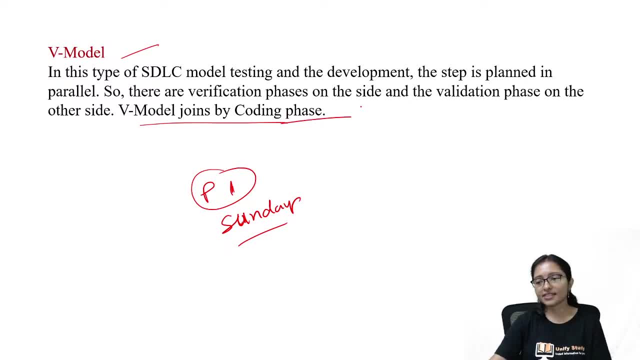 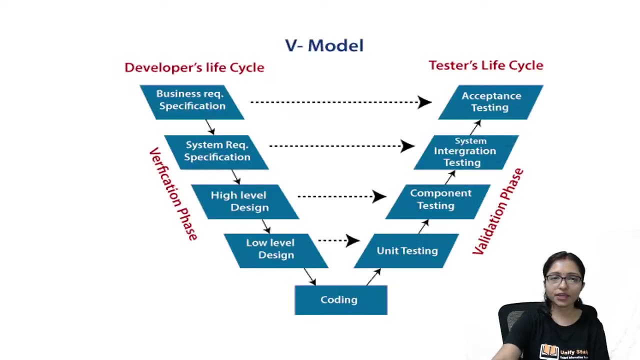 We model joined by coding phase here, Yes, surprise is coming, paper, one surprise is coming. so, as DLC model testing and development to stay planned in the parallel way here. here parallel way you can do that is the we model here developer life cycle verification phase are there and this is called the tester life cycle. both are working. 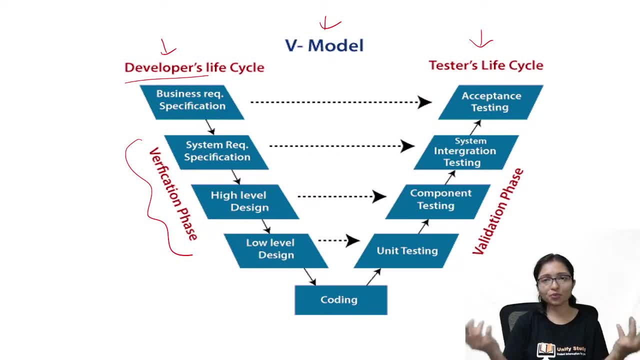 Parallely: Yes, Tomorrow, tomorrow, tomorrow maybe Five, thirty, five, thirty two, six or six PM. I will come with the surprise OK, tomorrow five, thirty PM or six PM. for paper one. I will come with the surprise OK tomorrow in evening time or maybe I can postpone this class also means I cannot, maybe I will not take the class. 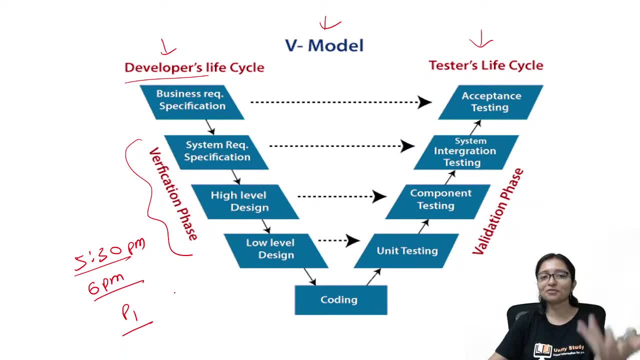 this software engineering class. at that time i can give you the planning of paper one and then then it will go ahead and paper one be ready for evening tomorrow evening. be ready, be ready for that surprise ticket. be ready within, say, after 5, 30 pm, any time we can come. 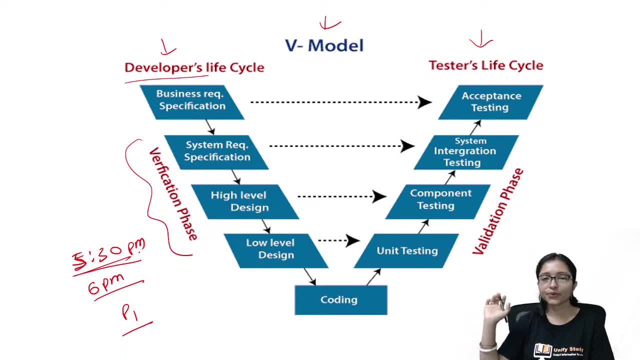 5- 30 pm. after that many time i can go live, okay. so we model check the v model. here. developer and tester are working together. developer and tester are working together here. verifications are there here. validations are there. okay, so business requirements system and all they will be there. 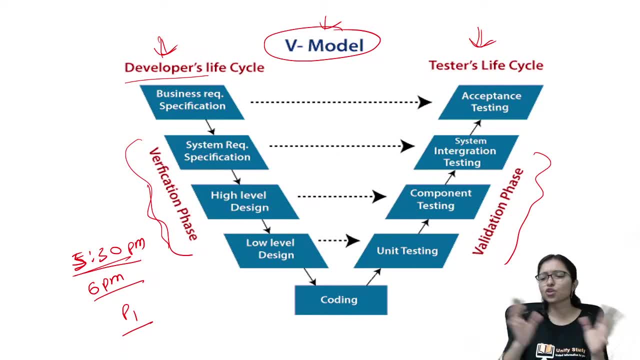 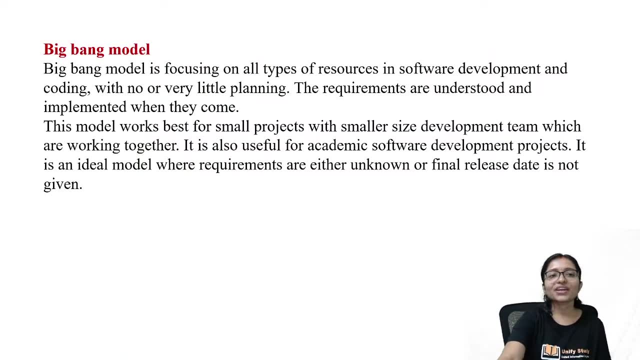 and after that that, each tester life cycle. that is, and that is it, the z Parte 1. c? r- no, that is it the case? no, then they. they only call v model. okay, yes, okay, okay, okay, now here, big bang model. there is another one. 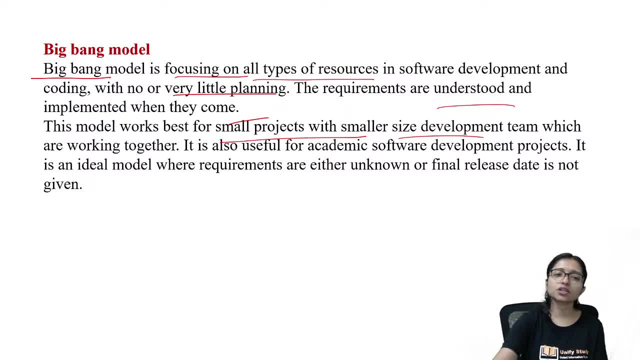 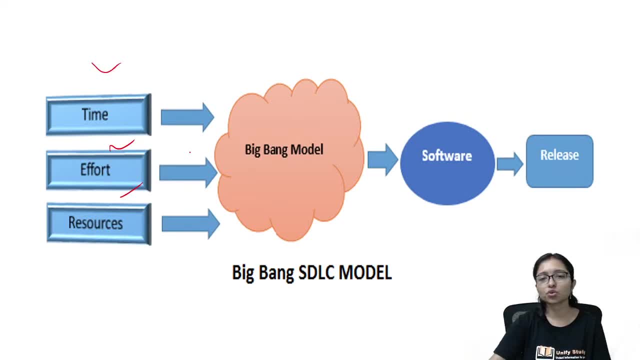 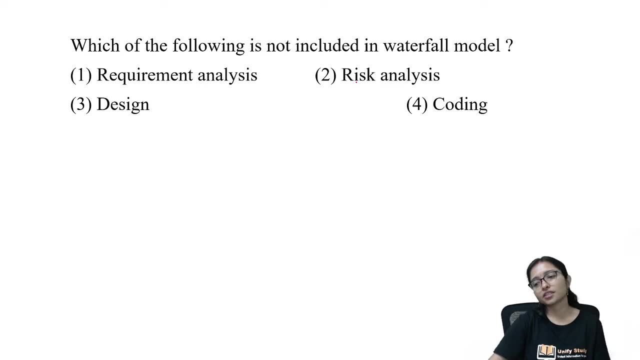 model- that is also big bang model, focusing on all types of resources and it's little, very. you can see, together you are doing everything: time, effort and resources. that is called the big bang model. as i tell me what will be the answer for this, notes i will upload today only. 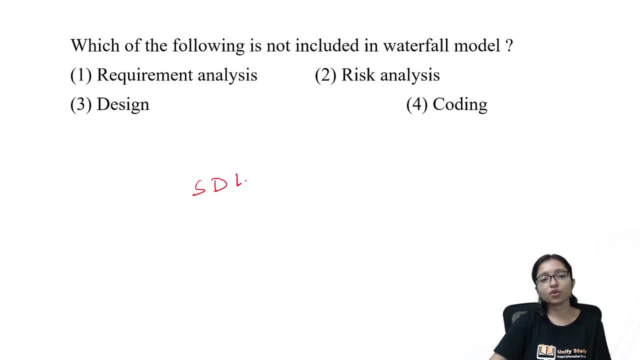 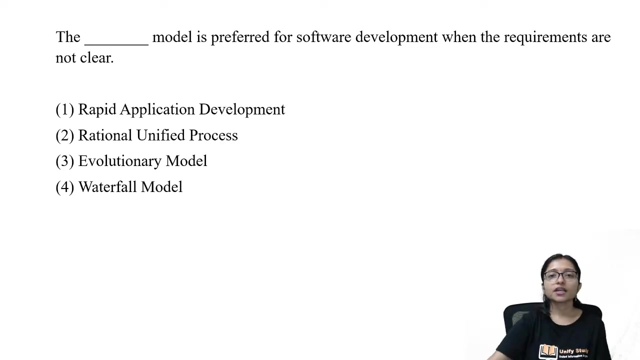 i will upload these notes. sdlc model note will be available after the class only. i will upload the note on unify study app. okay, difference between verification validation: we will do next class. we will do that. we will do that. do this one. yes, very good risk analysis is not there right now. do this one. 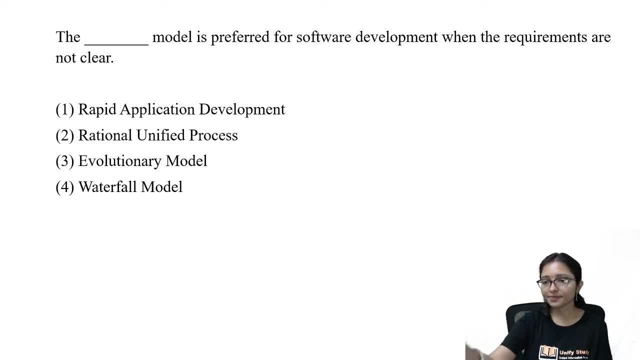 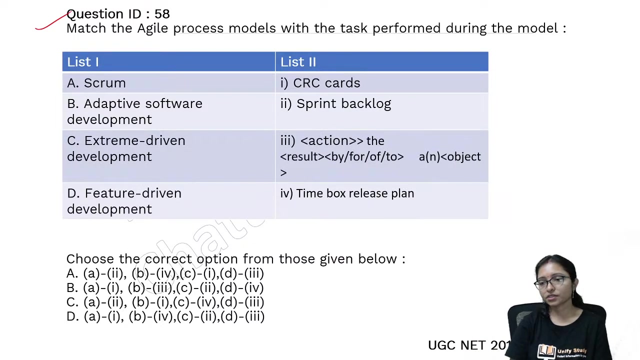 do this one. what will be the answer? the dash model is possible, preferred for software development when requirement are not clear. that is we did, this, is we did sorry. do this one, do this one, do this one. what will be the answer for this list? match the list. 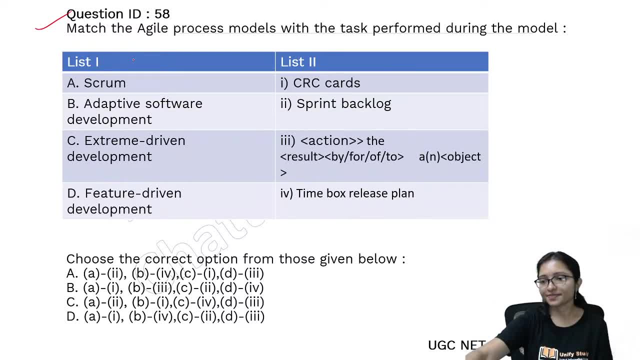 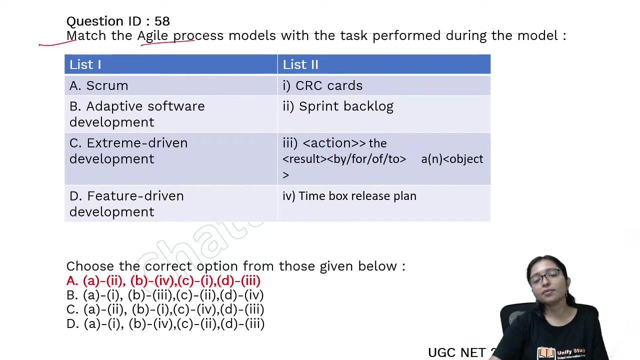 what will be the answer for this easy word? okay, all are giving answer. okay, so match the agile model. here you have to do the agile process in the scrum: adaptive software development, extreme debate development and feature driven development. these all are focusing agile methodology. but what are the different features that are given to the agile model? 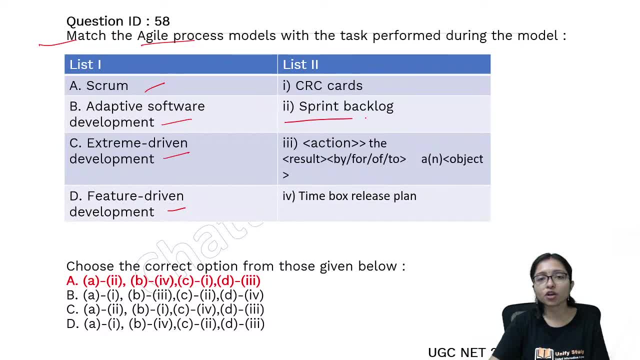 difference. so you can see the spreened backlog. spreened backlog where we are using the spring backlog, that is, in scrum. scrum is using the spring backlog. so a will be with two. this is not the answer. this is not the answer. adaptive software development. what they are using: time boxing. 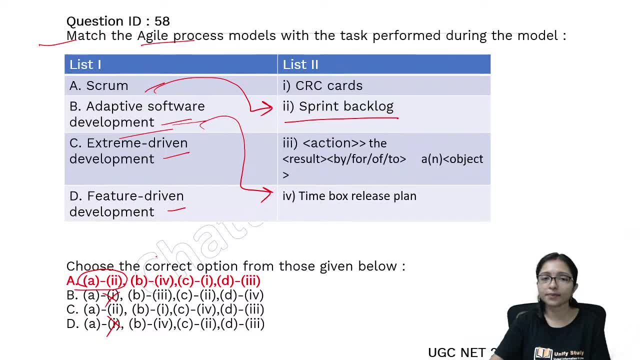 release. that is the adaptive software development. that's why we, with four extreme driven model is working on like action, result and object object oriented. feature driven model is. this is the sorry, this is crc card, it is working on that and feature driven model is like this. so that's why. 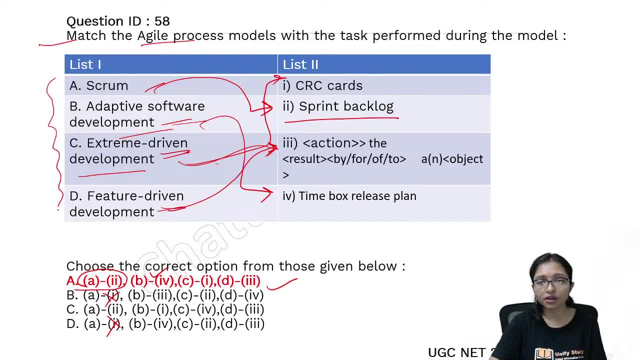 it is the answer must write down. these are the different, different types of development model: those who are focusing agile process model itself. they all are focusing on agile process model. okay, so option one is the correct answer, not option two or three. you all are telling what? option three to definitely not, option two, option two to definitely not here. this is the answer. 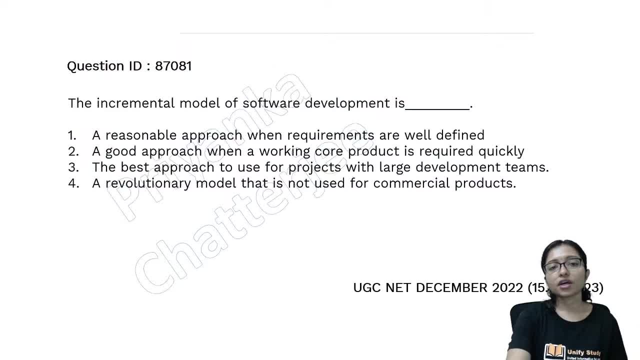 remember it, write it down in your notebook. so now do this one, do this one quickly, do this one quickly. the incremental model of software development is what? again you are telling mistake. the a reasonable approach. requirement are well defined. when requirement are well defined, you are telling mistake. again, you are telling. 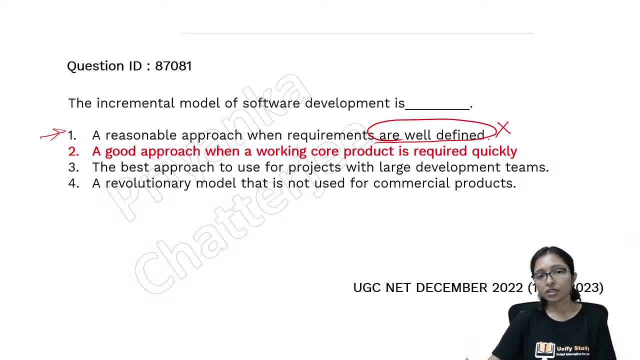 well defined, why we will go for it. the good approach. when the working core product is required quickly, core one you require quickly. after that, do the next one, very important. that's why we are going for incremental. incremental means the core one, the important one, give me. after that, do the 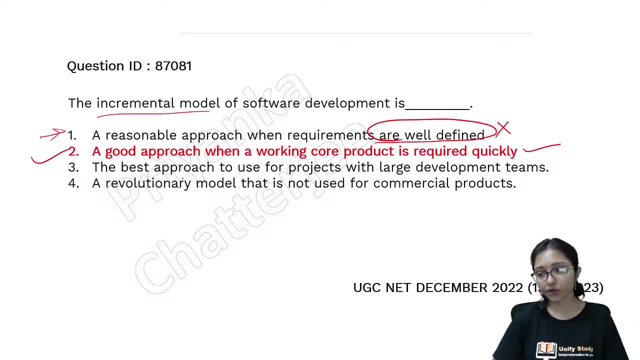 next one. then we will go for incremental model. right? yes, those who are telling three the best approach for use project, the large development. no, here, whenever it's required quickly, i have to give the core product. then we will go for incremental. now see that the model which required. 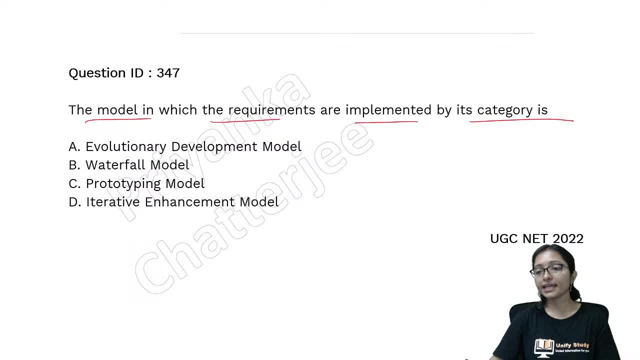 which implemented by category, by its category. what will be the answer for this? very easy to understand. we have no. the multiple application. yes, that is evolutionary development model, category wise. you are dividing that's by trees, society's etti development model. okay, it's not iterative. no, not prototype. evolutionary category wise you. 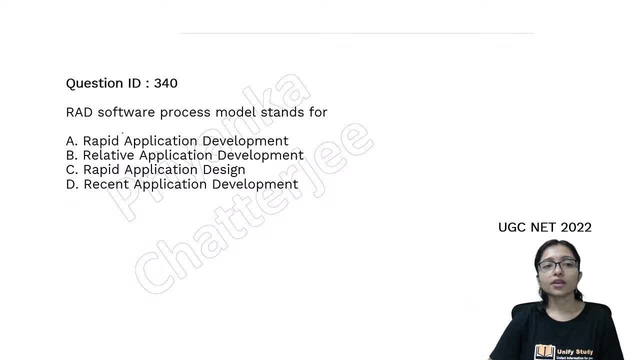 are dividing into part by part. okay, here you can see rad process model very easy. one is the best one. what is the rad stand for? so all types of mcq pyqs from everywhere? i asked you. i did, it is not only ugc net, from everywhere. i have collected all the types of sdlc model and i asked: 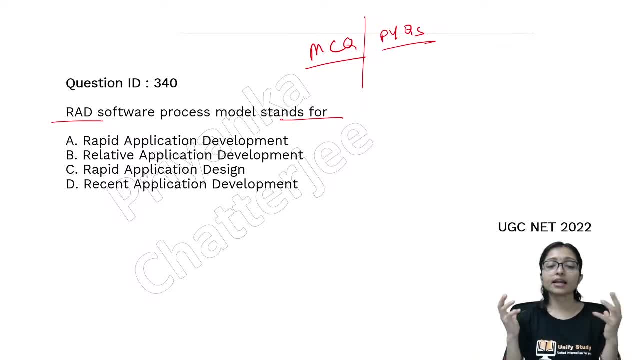 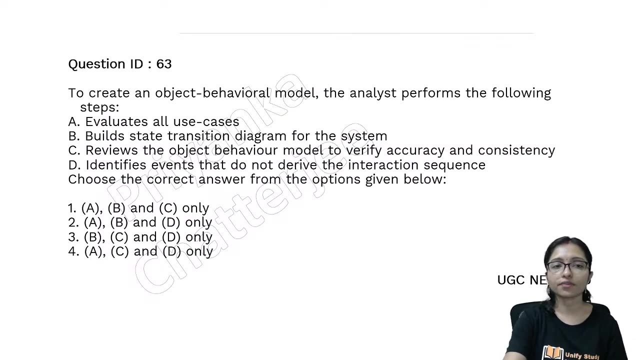 you the question we did. the chapter everyday class will be like that: i will try to provide you concept with the concept. we will practice the question also so that, completely, whatever you will learn, it will be complete. that is rapid development model. very good, everyone now do this. 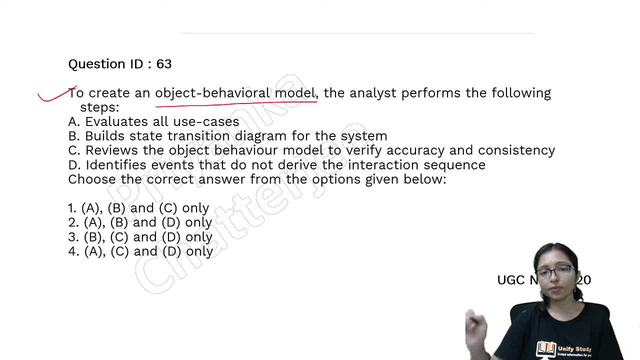 do this one, create an object behavioral model. this is one type of model. from the question only it will be clear: analyze, perform the following step in object behavioral model. this is also another model, actually in sdlc. so different, different types of models are there. different different models are there in object behavior. this is another model. 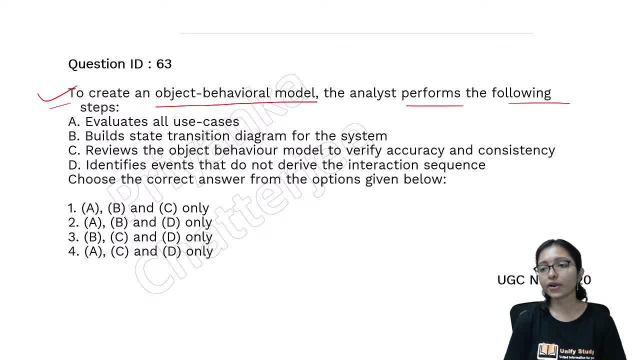 through the question. only it will be clear. you can write down the points from the question and from there you can follow it. that ます, simply watch me just soak. theで answer is here, so don't be afraid to follow the example. it is very easy when you do so. 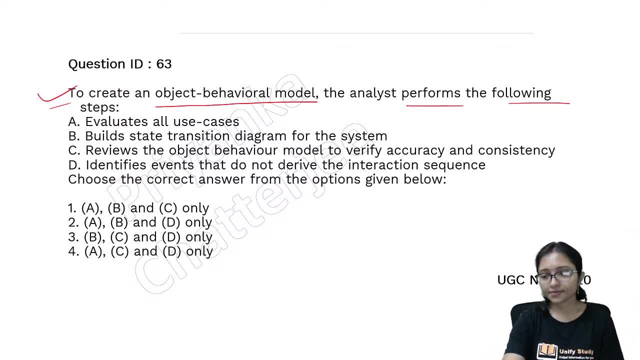 toief. both use your aux pressed Option 1, evaluate all use cases, build the state transition diagram and review the object behavioral model because it is object oriented, so object behavioral is should be there. so option C should be there here, no option C here. option C is here here option C is there, but here you can see that the these are the three main feature. identify the event, do not derive. 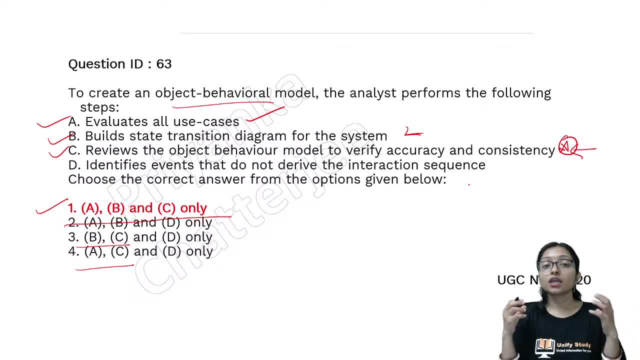 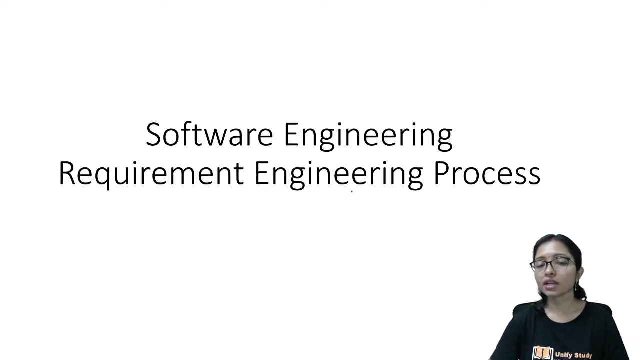 the interaction sequence. so sequence diagram, use case diagram: we will learn. we will learn that in the design part. what is use case diagram, what is sequence diagram, what is class diagram? I am going to teach that also, so for now you can write down in your notebook: these are the three main feature of object behavioral model. okay, yes, so next class we will do this chapter. this is also next important. 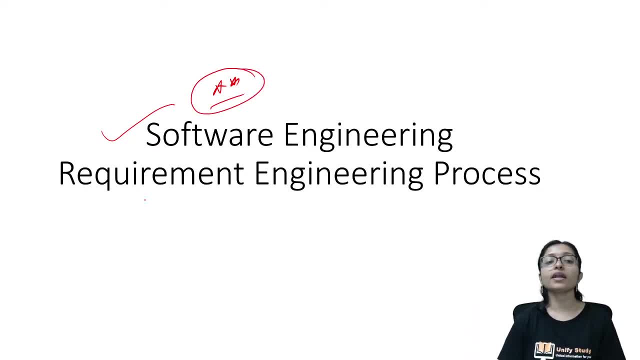 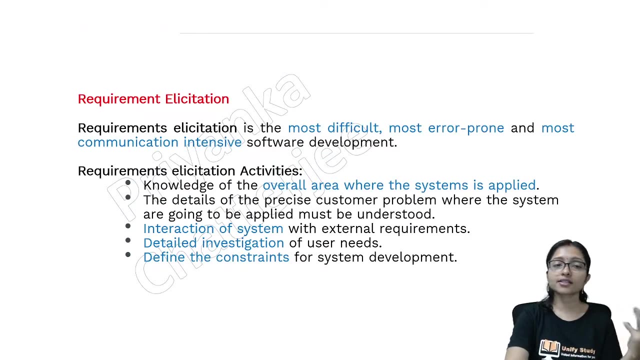 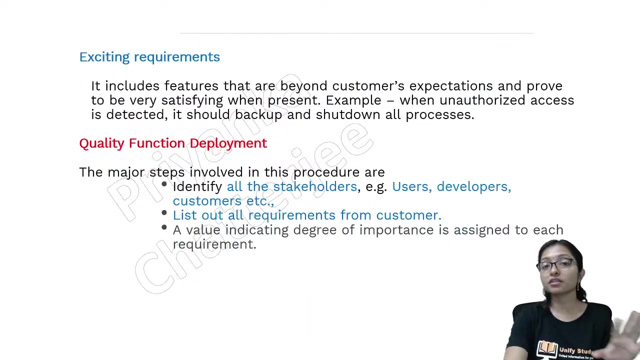 chapter very, very important from here. frequently they are asking question: software requirement, engineering process. this is the things we are going to learn in the next class. so many concepts are there. this is very, very important: concept of characteristics, SRAs and all these. all the things we are going to learn in the next class. so come to the next class to learn these all. okay, I will teach you like industry standard only, so be careful.